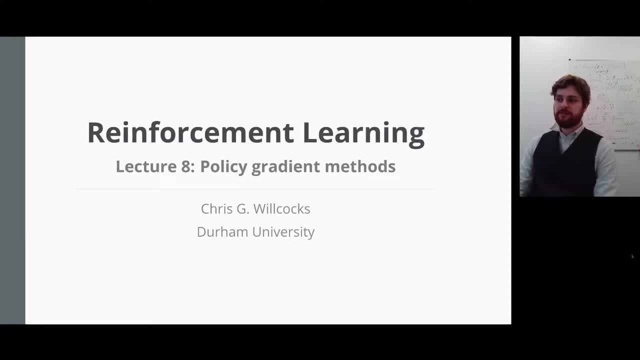 And today we're also going to be using function approximators. but we're going to be trying to learn to characterize the behavior of an agent, So the policy of an agent or some distribution over the actions it takes, conditional on being in some state, So it can be like a lazy agent or 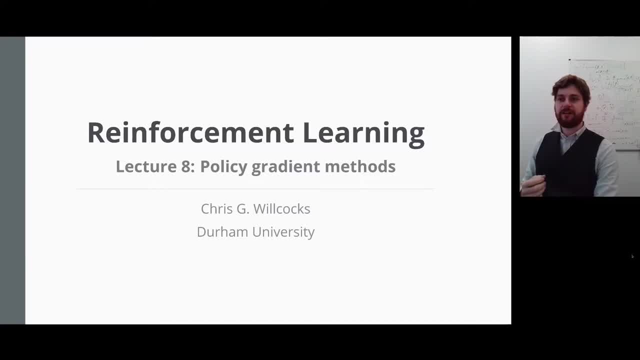 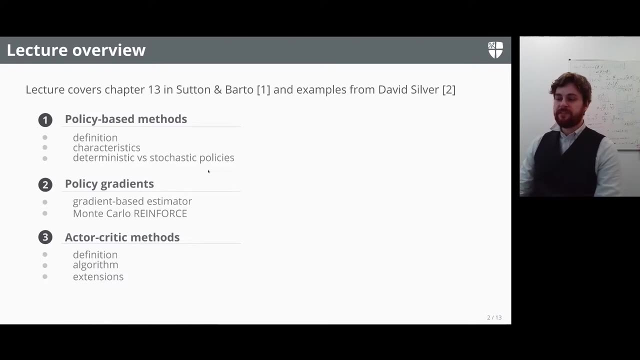 a hard-working agent and we're going to try and parameterize how it should behave, or whether it should be lazy or whether it should be hard-working, and what is the best policy to do So. in this lecture, I'll introduce policy-based methods and we'll discuss their various 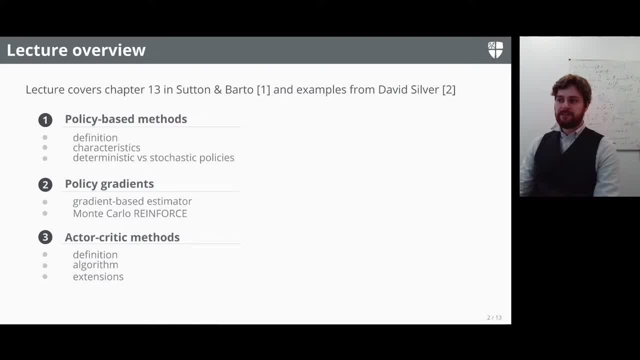 characteristics. In particular, we'll look at their advantages and how they can give better convergence guarantees and work in continuous action spaces, like, for example, controlling a robot, and we'll examine how they can learn stochastic policies, which are especially advantageous when using value function approximators or, in particular, in partially observable environments where you can't quite see the 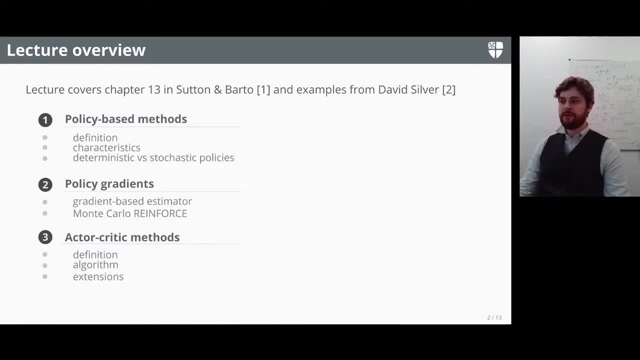 entire state space. You can't see the whole environment available to you, again like if you're driving around in a car. you can't see all of the contents inside the building. so you've got this partially observable environment, And so these kind of approaches work particularly well. 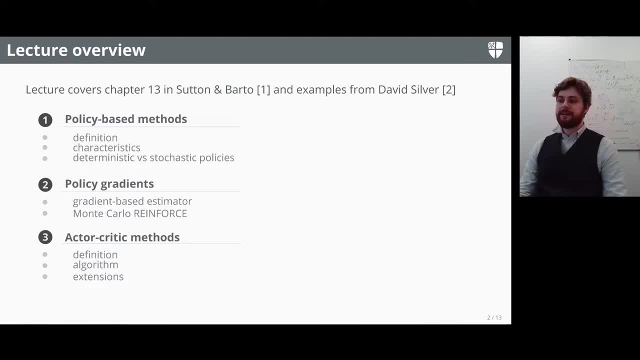 in that case. And then we're going to look at the definition of, say, just policy gradient estimators, how we go about optimizing the parameters of a policy function, and this will lead us nicely into the reinforced algorithm, which is quite an old algorithm, but it's useful to lay a foundation down. 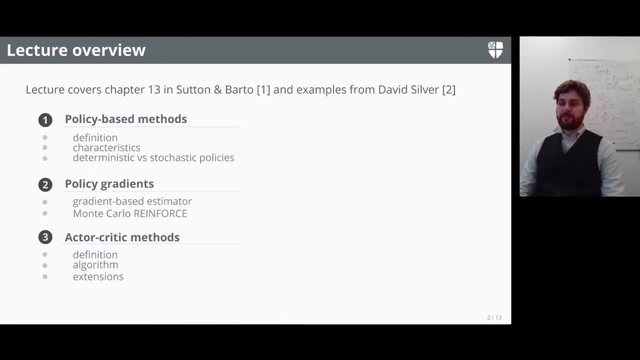 We'll be spending the last third of the lecture on more recent methods, specifically on actor-critic methods, and these are where you have two neural networks: One is the actor, which chooses the actions that you take, and the other is the action that you take and the action that you take and the 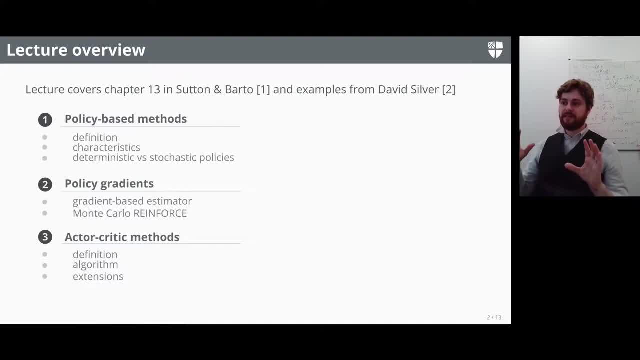 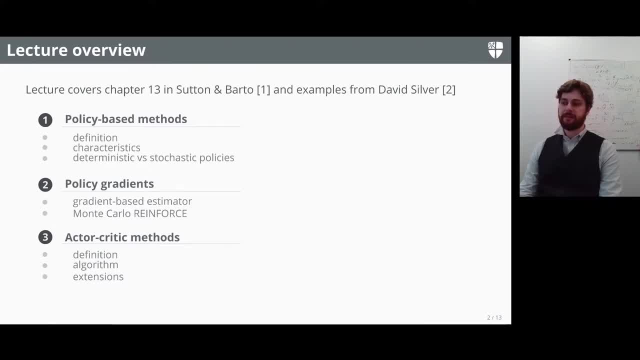 some kind of extensions where I'll outline some recommended further reading that builds on this. so this will be like a foundation, where you don't got the tools available to go and read the state-of-the-art papers and go ahead and implement more advanced techniques. These are 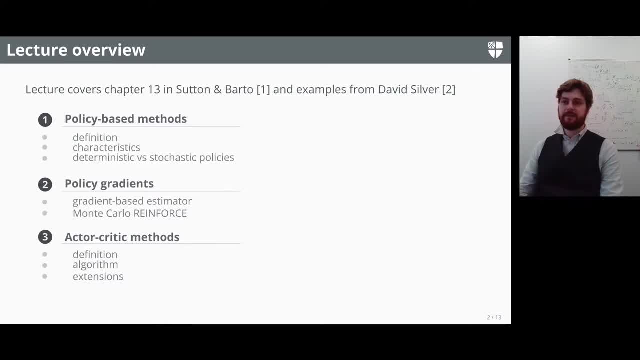 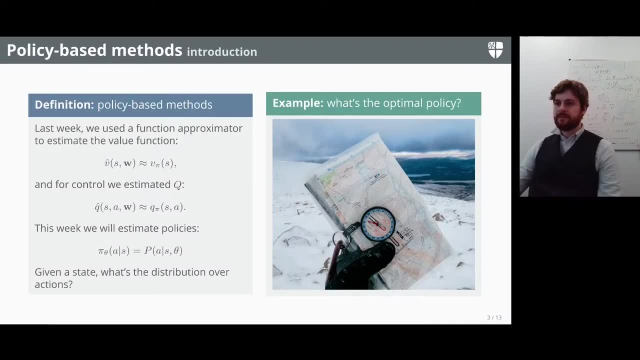 going to be particularly relevant for scaling these methods up and doing more complex environments, like you get in the assignment. Okay, so in the last lecture we considered two types of value function approximation. We parameterized the function by some weights vector, so we we had this approximate. 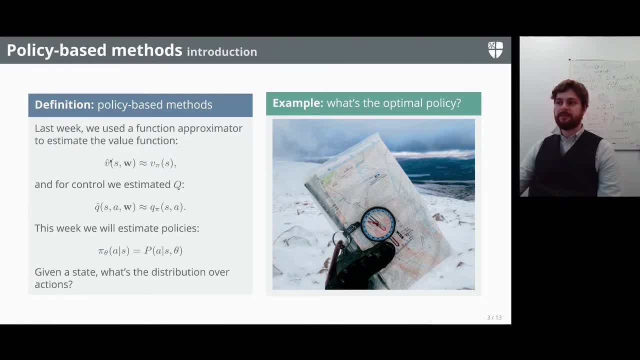 approximation of the weights vector, where we considered the state value function, which which tells us how much reward we get from some MDP in expectation if we follow some policy. this this pi. So if we're in a state, the function tries to estimate the expected value of the reward. 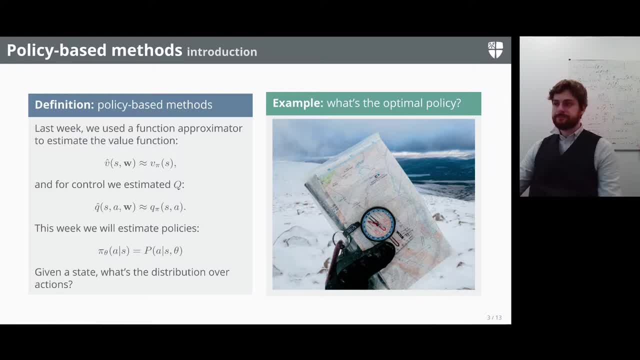 we'll get from that point onwards under under that policy. Then we discussed the, the action value and the order, if you like, the q function. This tells us the true accumulated expected reward we can get from being in that state and taking some action. a again under under that policy, pi. 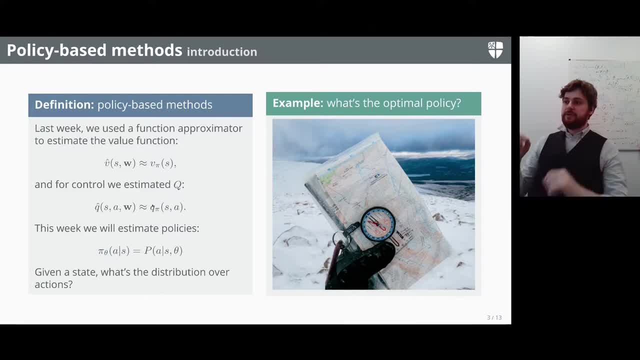 And what we did was, instead of storing like a massive table, or this big table for all of the action values, we used a function approximator, like a deep neural network parameterized by the weights vector w, to approximate all of those values. So the inputs to the neural network were the state and the action being considered: the state and the action. 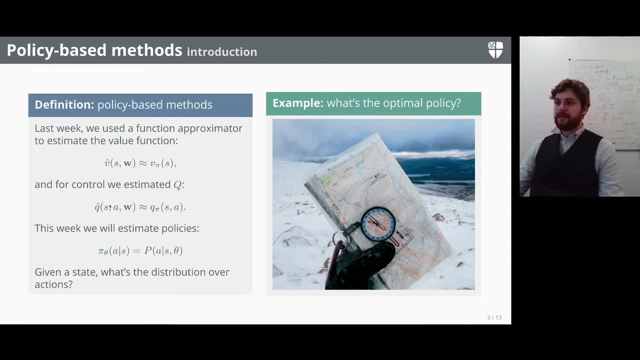 being considered and it would basically try to estimate the value of being in that state, And that's that's not always the best idea, like if you're in a complicated environment, to try and work out the whole value that you would get from all of those future actions can. 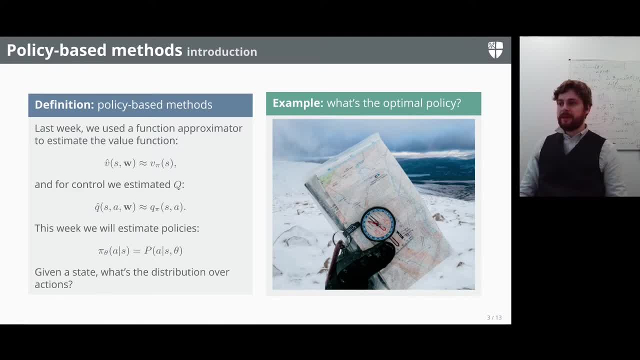 actually be quite a difficult thing to do But nevertheless we we treated this like it was a supervised learning problem, where we started off trying to estimate the value function and we took a max over all the actions and used that as our ground truth. And, if you remember, we saw that this had some kind of convergence issues, which we some was. 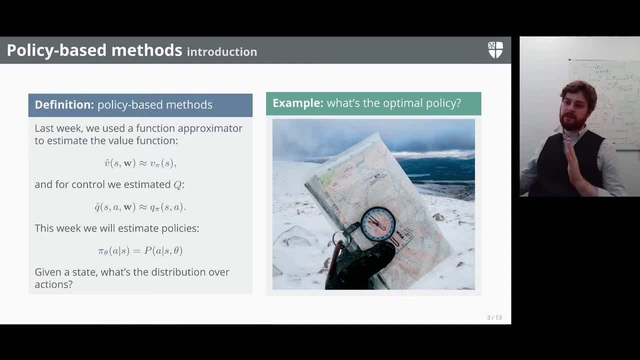 addressed by aggregating all of those experiences that you receive when you play the game into into and that helped create like a kind of mini data set, if you like. that was less susceptible to the episodic correlations and issues of it being non-iid, so it helped, but it, but it. 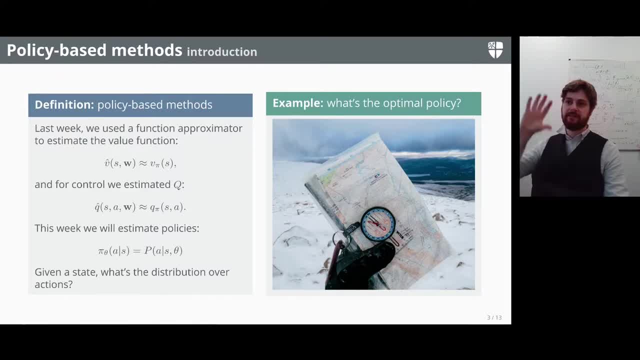 but it still had a few issues with it. but it does greatly stabilize it using those kind of replay buffers. and we also looked at more advanced strategies like important sampling, where we weight the experiences we receive so we don't just uniformly sample from that data set. 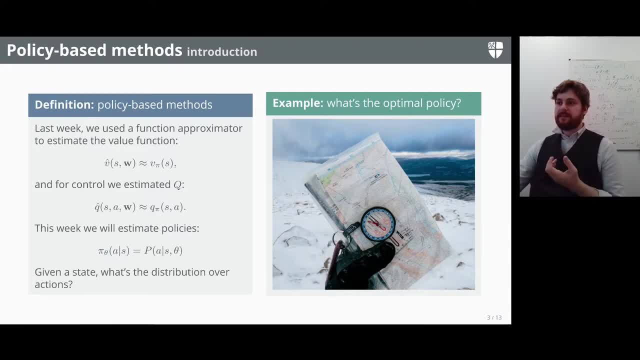 Okay, so what has been the policy itself, as we've been? you know, if we go back through all of the past lectures, what has actually been the policy we've been learning so far? Well, with all the techniques we've been considering, we didn't really have a notation of a policy function. 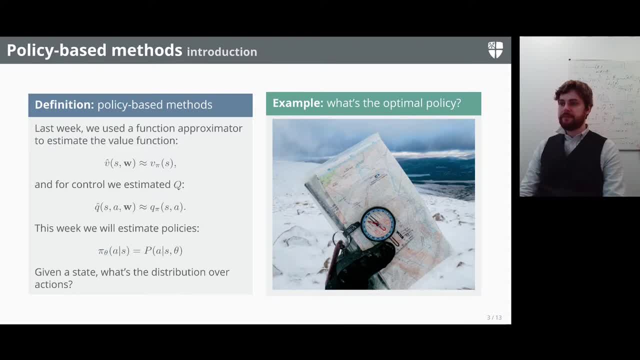 maybe at the very beginning we briefly touched on it. but in other words, the policy hasn't really been explicitly represented before and we've just said that we optimized the policy by taking some over our action value functions. so we find the action that has the, that maximizes the reward. 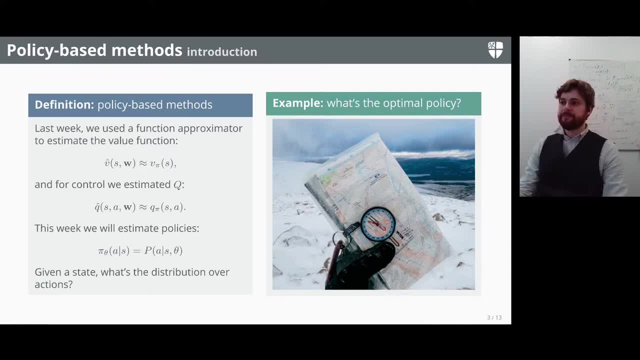 and we say that that one, there is our policy. so we just acted greedily, or epsilon greedily, as our strategy to find the best policy. but now what we're going to do is we're going to have a different approach where we're going to have a different function: approximator that parameterized. 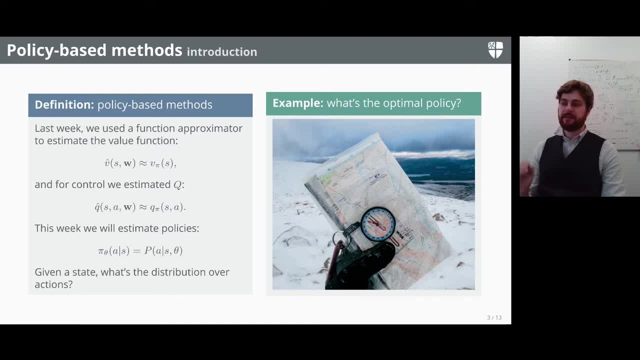 the distribution of actions conditional of being in some state. so we say that the parameters are represented by some vector, theta in this case. so last, last week we had w as our our parameters and this week we're going to be looking at theta and we're going to change the parameters. but if just 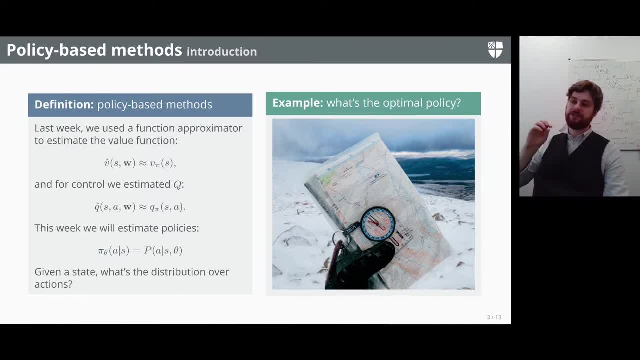 imagine changing those parameters. that's actually going to affect the distribution over which actions we take or which actions are chosen. so instead of choosing the maximum action, we're going to be sampling from a distribution of actions. so if we look at this equation down here, we say: 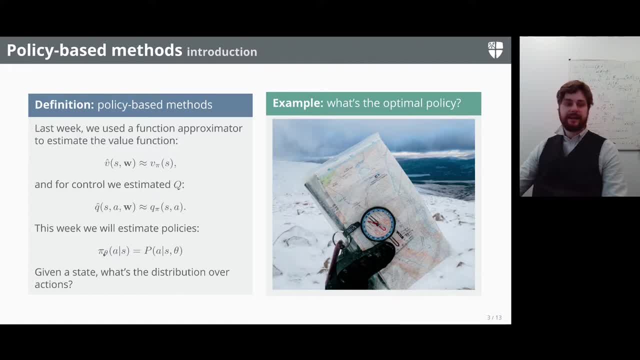 that the action a is the probability that the action a, given the environment, is in the state s so and it's parameterized by theta. so you could also notate this with subscripts on the variables. eg to say this occurs at some time, step t. you could say action t or state at some time, step t. 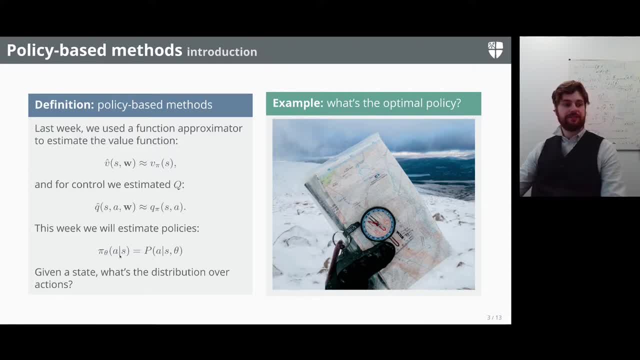 but basically that's what it is. this is the distribution over the actions conditional of being in some state, and i hope that's kind of clear. today we're going to be looking at how we can optimize within this kind of framework and it is worth mentioning that this all kind of deviates quite a bit from what we've been studying. 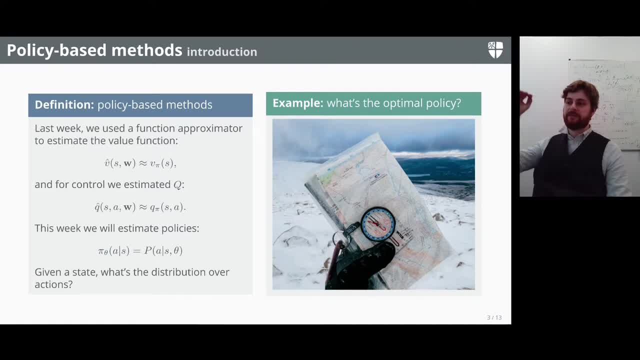 so far. so everything up to this point has been layering methods on top of the foundations, but today we're kind of going to go off in a bit of a tangent. basically, this gives us a distribution of actions that we can sample from. so, instead of taking that maximum, we can sample from this. 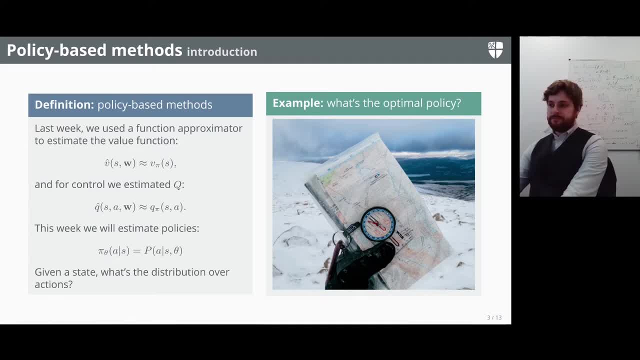 probability distribution, and remember the p here is kind of like: this is a probability mass function or a discrete distribution, but it could also be like a lower case p for a continuous distribution, so we can actually learn to sample from continuous action spaces, right. so why might we do this? well, sometimes. 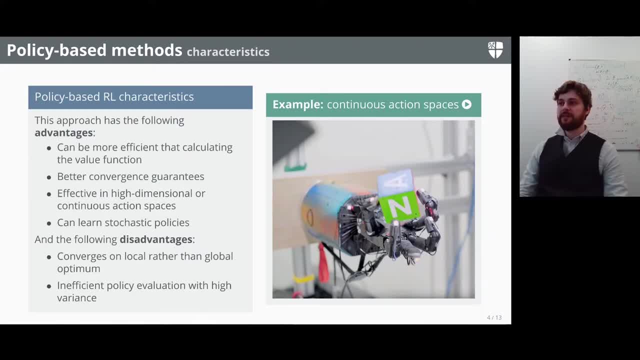 it's more efficient to represent the policy than it is to represent the value function. so consider, for example, like one of those atari games, or let's just think specifically about the coursework for graphics, or something like that. so let's just think specifically about the coursework for. 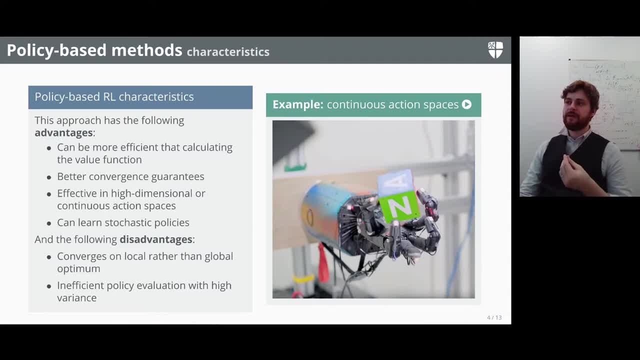 gravatar um. consider the value function. it might be very difficult to work out what is the expected. value is, from some point onwards, based on how much you rotate your ship. so it's like if i rotate my ship to the right, what is if i play optimally throughout the entire game? what is the most? 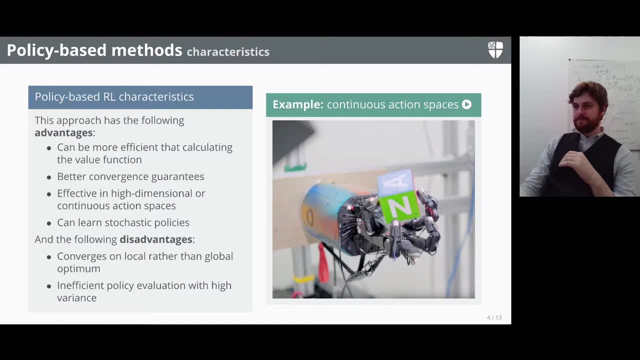 score. i could get having that as your value function and that's like really really hard because, um, it's like playing the game tetris: it's really very difficult to work out like what your score is going to be, given that you move left or right. you might know that is that you can improve your score slightly. 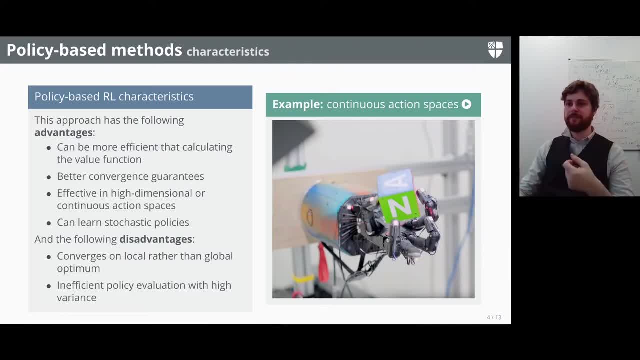 or do better, or it's not good to let the ball fall down, but it's very hard to work out the total reward you'll get going off into the future. so, um, if we go back to gravatar, you know if you've got a wall in front of you and you're about to crash. it may be quite a simple. that might be a. 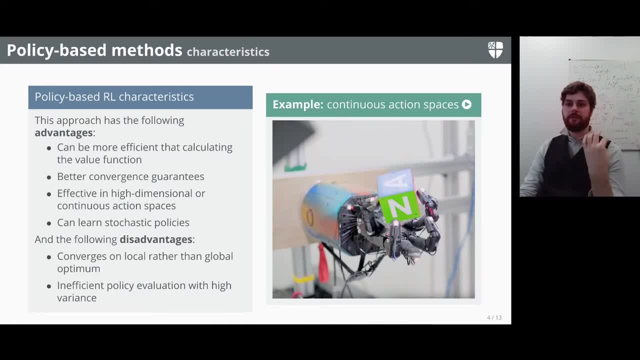 simple policy which just says: turn around and move away from the wall. you know that's quite a simple thing to parameterize and that's much easier than working out that you're going to get a value of, say, 532 points if you hit the wall, versus 619 points if you don't hit the wall. 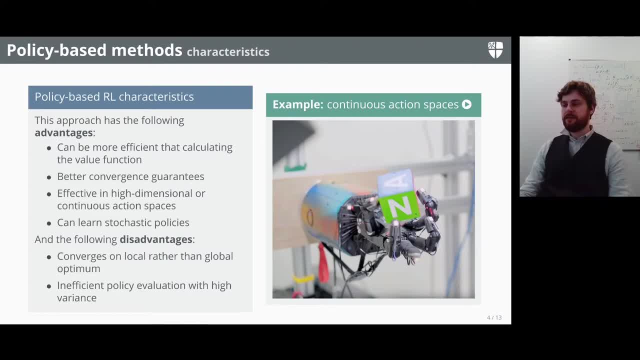 so, similarly, if you remember back to the last lecture, we had all of those issues of convergence with dqn's dq networks and we needed to start doing several tricks to make it all much more stable. and do you remember we had those cases where it would have been. you have those catastrophic 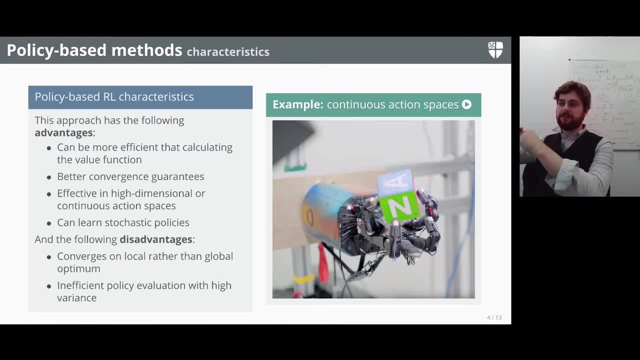 divergences can occur and you get those chattering around the value function. so we started to add: like learning strategies with experience replay well income. in contrast, if you follow the gradient of your policy, you tend to smoothen out the policy, which leads to increased stability in particular. 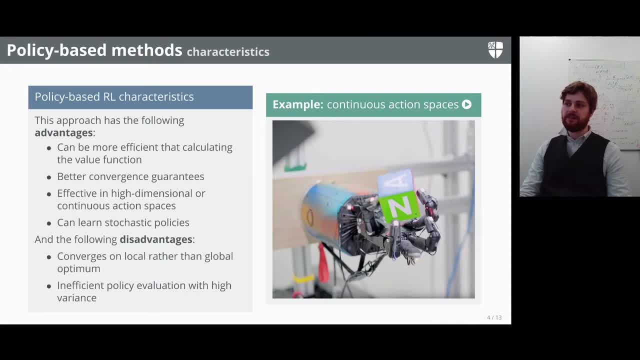 you don't kind of tend to see those catastrophic divergences that you get and you tend to always find at least a local optima. so this all becomes much more like classical deep learning, where you've got some kind of bias, variance, trade-off based on the parameterization and the regularization. 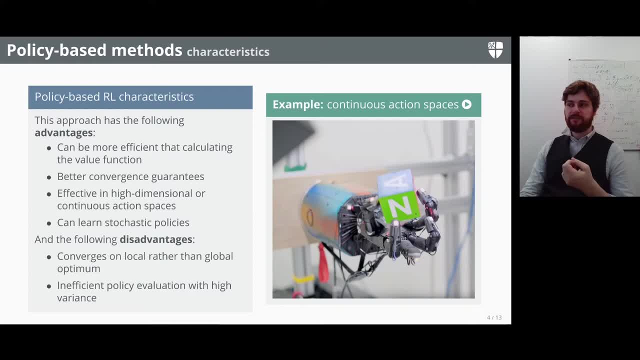 and policy-based methods also tend to be quite effective in high dimensional or continuous action spaces. so remember, with the value-based methods or the action value-based methods, you need to act greedily over your actions. so you need to compute, like that max over the set of actions. well, while that's been quite easy, what happens if you say you had? 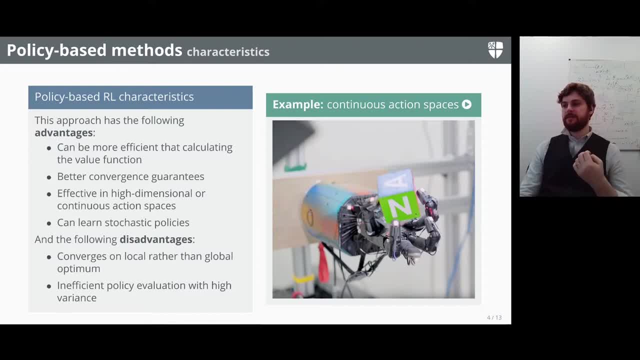 trillions of possible actions available, or even like an infinite space of actions, like an infinite number of actions. for example, if you're controlling the robot robotic arm in this figure here, then you know you might be able to change the voltages of the signals in the actual actuators. 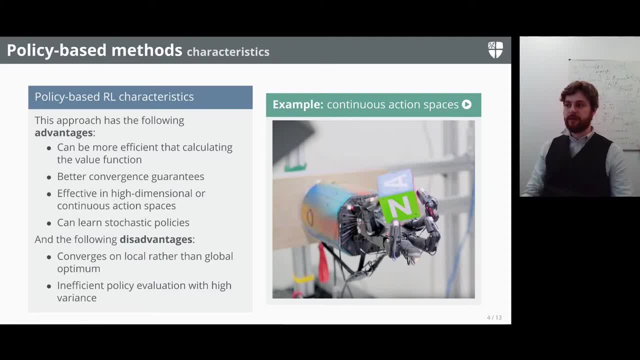 and this voltage might be an action represented as a real number. so you could- you can have an infinite number of voltages to, to move and expand the fingers out, so it's not like you just choose to move one of the fingers discreetly. so how are you going to do a max over that like? 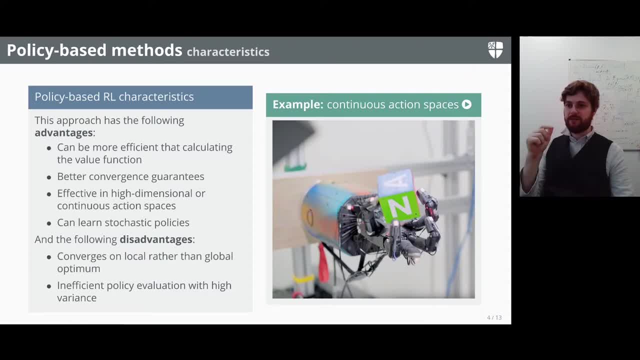 you've got like millions of possible voltages you can put into all of the different actuators to work out. how are you going to just take some max to find out what the optimal voltage is? or you consider like discretizing your space into some very, very large, large number of possible? 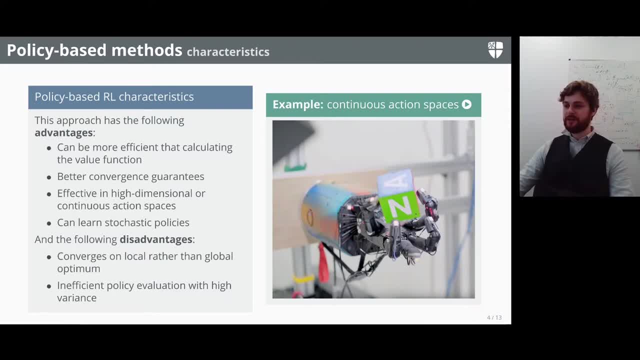 discrete settings that are still going to be super inefficient and there are cases or environments where you just can't easily do it. you can't take that max, that that max becomes intractable. so instead you can use this policy-based method where you adjust all your parameters to learn. 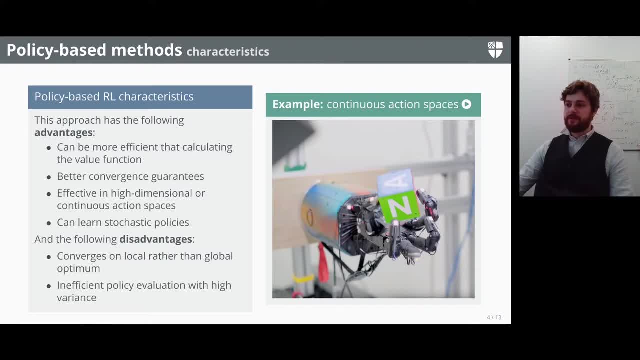 your policy directly, so where you start to learn what the max likelihood might be, rather than just having to explicitly compute that max. and this leads us really nicely onto the fourth reason why policy gradient methods are advantageous, which is that they can be used to learn stochastic policies. 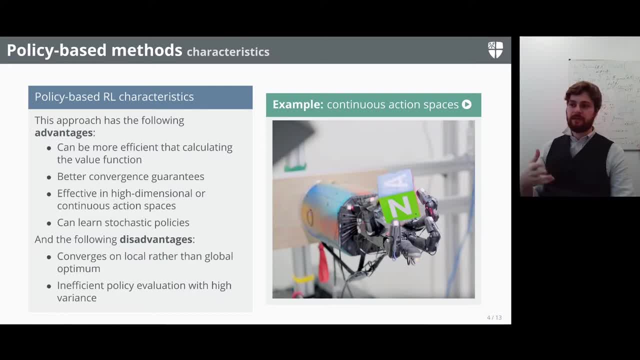 as opposed to deterministic policies, and we'll see why this is very important in the next slide. but it's also mentioned there are some disadvantages to this. it's not just like a win-win, so naive policy-based learning can actually be a bit slow and it can have 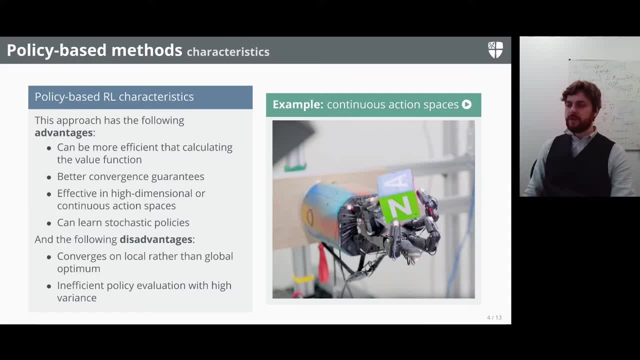 higher variances than value-based learning and if you think of value-based methods, that max, if you like, is very aggressive and always moves directly to the mode of the distribution and it it tends to find a global optimum when you, when you take that max, which is really good. 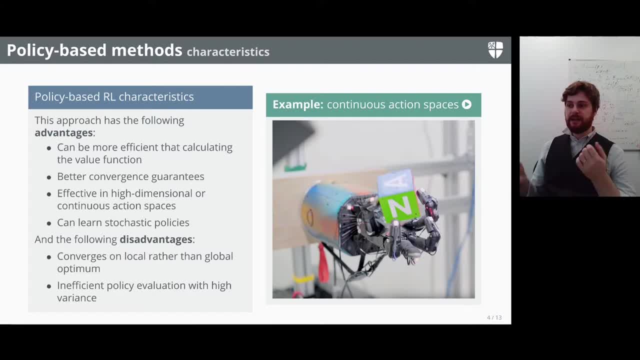 in theory but in practice. remember that in deep learning we often want to find like a good local minimum that generalizes well. well, policy-based learning tends to find a good local minima rather than like the global optima, which means that it can often get stuck doing quite. 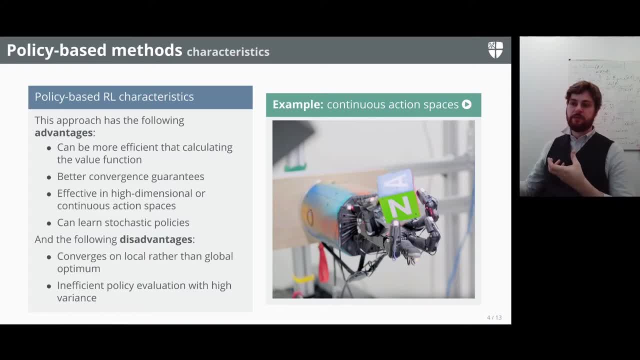 sensible things, but it may not find rare cases of optimal behavior. so if if you're like stuck in this maze and like most of the paths lead forward and you know your goal's in that direction, so on the expected case, it would be sensible to move towards the goal. but it might be that there's 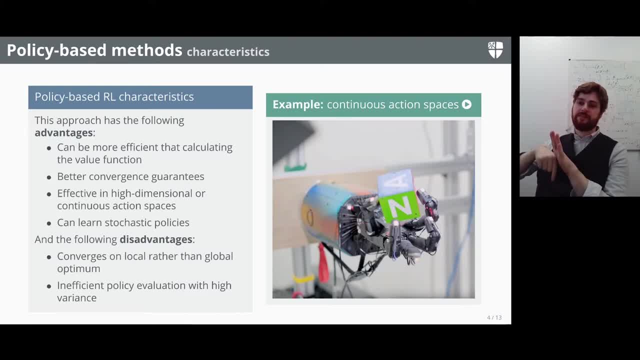 this rare strategy to go backwards in the wrong direction, into this really small, obscure door which goes on this really really long, complicated tangent but actually ends up being faster than go at taking an immediately obvious path to take. So they tend to get stuck doing these sensible. 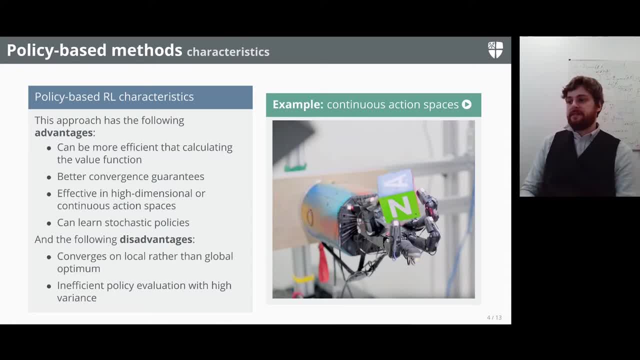 things and you might, in rare cases, not find this optimal behavior that you might find otherwise if you were to take the max. So this is all because policy-based methods learn a distribution over the actions, eg a softmax function. so it's a lot smoother in practice and to learn this distribution. 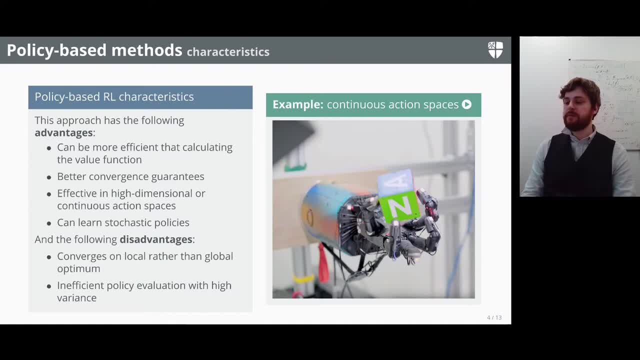 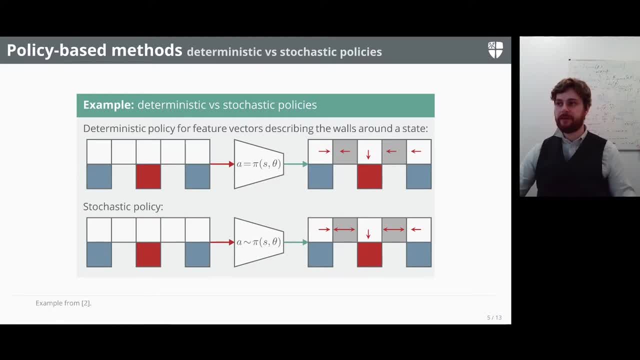 Okay, so this is an example that I like from David Silver, which helps explain why stochastic policies are particularly important with function approximators. So, looking at the top left here, imagine we have some small grid world like you've seen before and just like before you know it's. 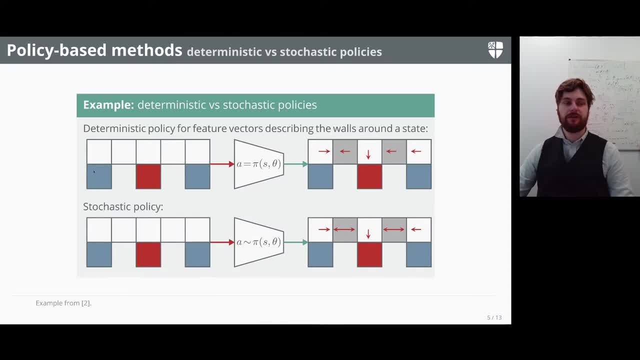 like this frisbee game where if you fall into the melted water you terminate and you lose, but if you manage to move around to find where the frisbee is, then that's that you get some reward and that's a good thing. that's the correct state to find. 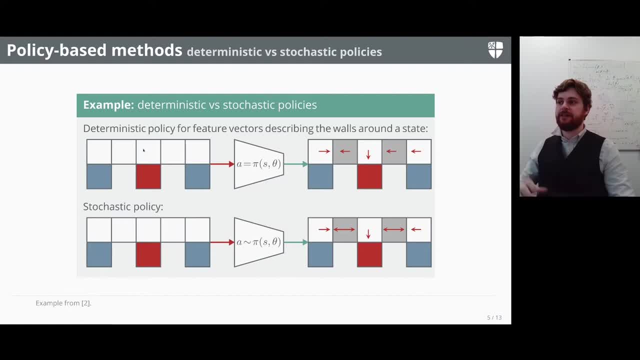 But try to imagine this as being like some infinitely large grid world where you've got some infinite number of states, like it could be this kind of continuous action space- sorry, this continuous state space, like in the real world, where we can move in many, many, many different positions. So instead we're going to try to 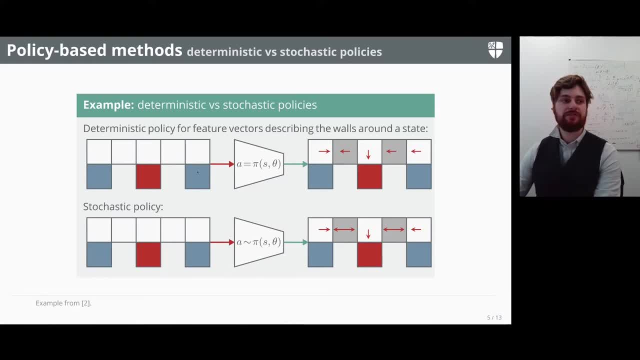 imagine that these are like stochastic two grid world's. you know you're not having like every state represented in some table, so just try to imagine these states are estimated by some neural network. so the neural network looks at the state locally and it tries to represent it by some. 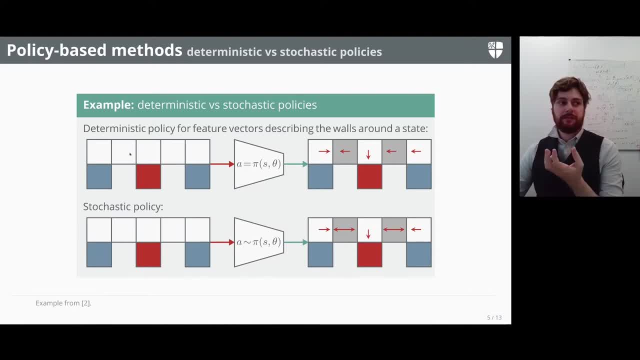 feature representation. So we're going to say there's some network out there which takes as input some local conditions of the state and it estimates the feature that it's in Well and so the features you might just say, like having a wall on the left above to the 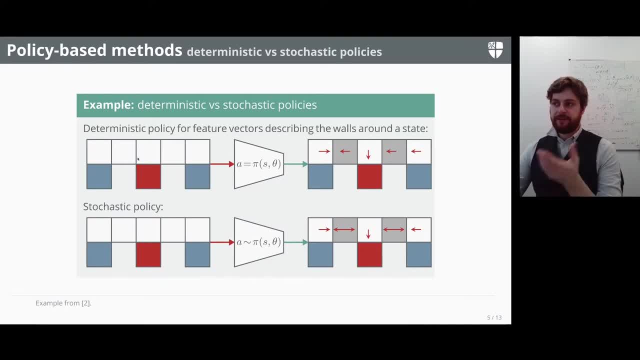 right, so on that there are feature factors. so specifically we're gonna say the far left wall here is distinguishable as we've got this wall to the left. and the far right state here is distinguishable as it's got a wall to the right, and then the middle state. here we can say it's distinguishable as it's. 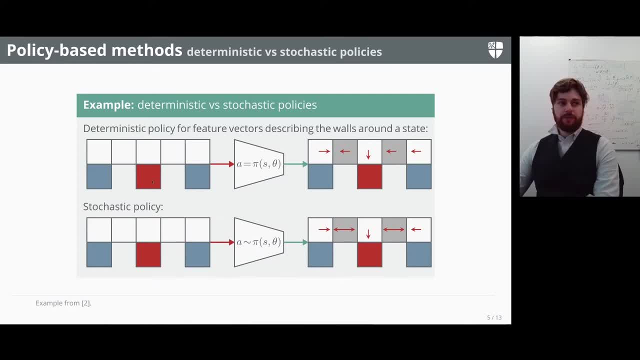 got no walls to the bottom here. you know you can walk from here into this state here, but then the other two states here, or this state here and this state here, and they're indistinguishable from each other, or locally they look the same as each other because they've both got walls on the top and the bottom, but they 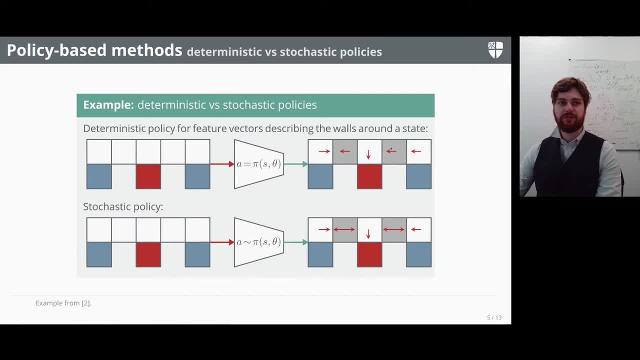 don't have walls on the left and the right because you can move between the states. so these two states, according to our neural network, look identical to each other within this feature representation at the neural networks land. so if we were to actually follow a deterministic policy function which chooses the action simply based on the input features and 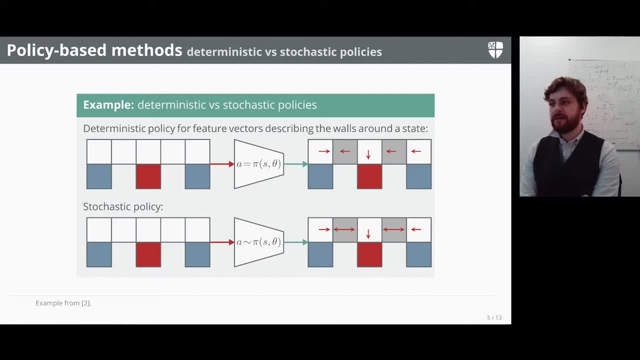 we then choose a max over action based on it, then we'll get the same value shared across both feature representations for this for these two states, because they locally look identical to each other. so this means that a deterministic policy function will have to choose the same action in. 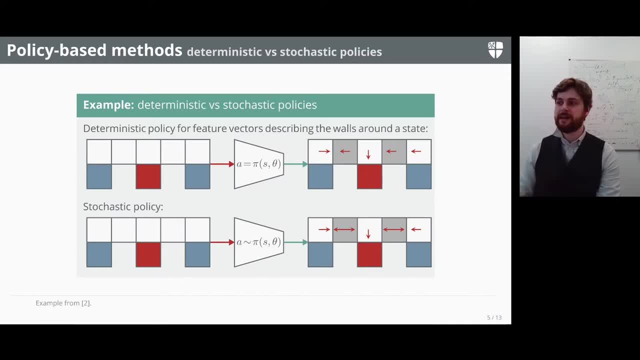 both of those states, which means if you were to act greedily with respect to this value function or the action value function. it means you're either going to go left all of the time or you have to go right all the time, and in this case we're just showing that you have to go left, as shown here, and that means you're. 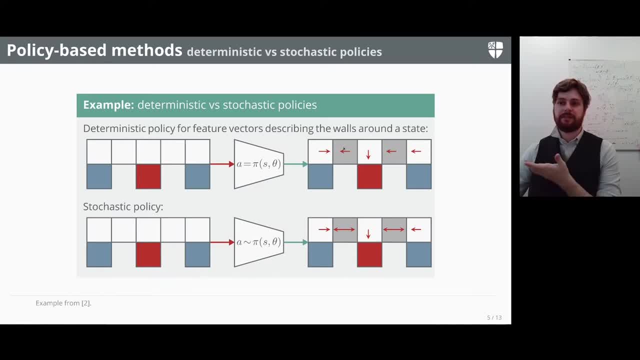 going to get stuck in some local minima and it's never going to converge, no matter how many iterations you do. so if you're in this state here, you're always going to go back backwards and you're never going to be able to get out of. 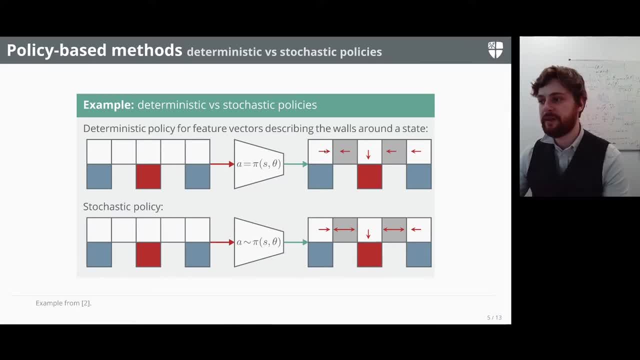 this, this local minima here doesn't matter how much, how many times you iterate that, but if we use this, learn to stochastic policy, so we, if we learn to sample from this policy here, let's learn some distribution over our actions. this means that we can encounter a feature representation which is shared across. 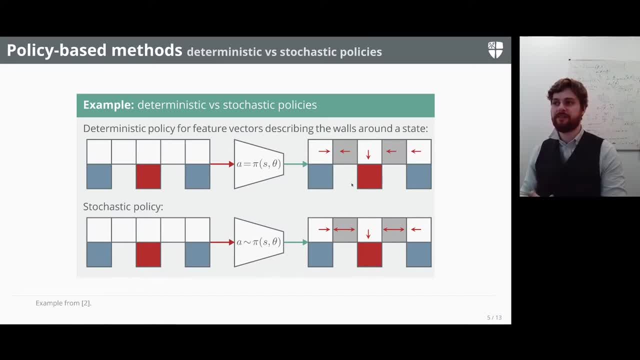 many states we can actually capture the value of that feature representation as a distribution over which actions should be taken. so in this case there's walls above and there's walls below, but there's no walls to the sides, just like in these two states. we can basically learn to move either left or right with 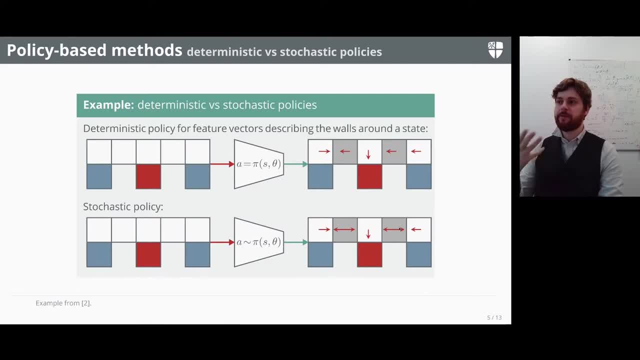 equal probability and therefore when we explore around we're not going to get stuck in that local minima in this far left state, because it will have some equal probability of going right or left. so some of the time it will come out of this state and move correctly down, and similarly here some of the time it will. 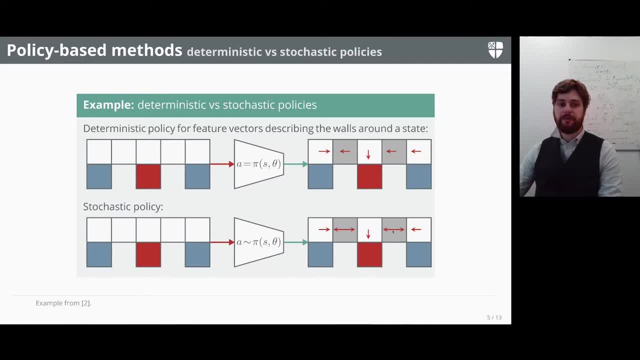 some of the time it will go back again, but some of the time it will move out of this state in the correct direction and come back down again. so that's much better because it means we don't get stuck into these local minima and we will eventually find those nice high reward situations. 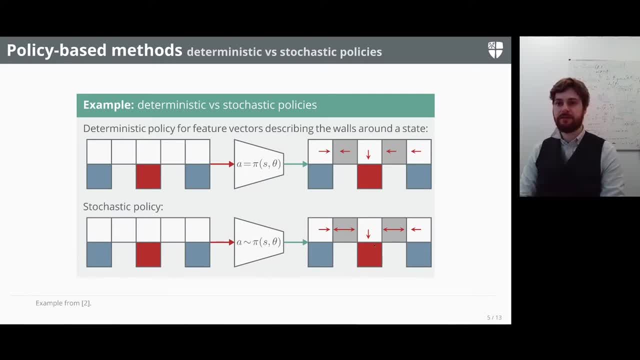 even even though the states locally look the same according to our feature representation. so you may be a little bit confused at this point and remember something we said early on, which was that there's always a deterministic optimal policy when you have an MDP. but you've got to remember that was for a 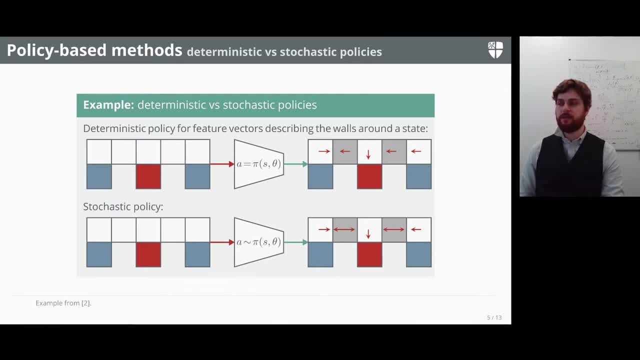 complete Markov decision process or a complete MDP where we stored the value function in this large table and we have this perfect state representation. but what we have- is a part is often have- is partial observability, where the features you want from your function- approximator- limit the view of the world or they 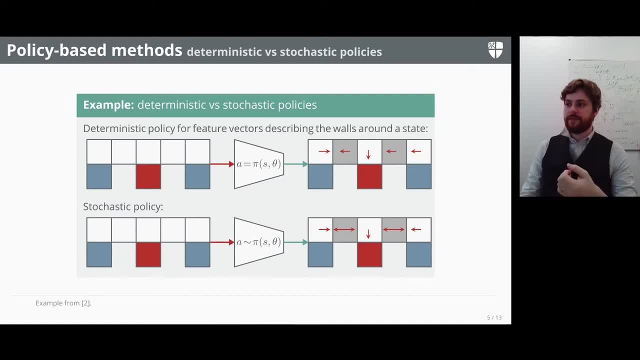 limit what you can experience, see visually, and then it can be optimal to use a stochastic policy in these cases. so you can imagine a state in a game where it looks the same as some other state, but actually you're in just based on your experiences. you're actually in very different pictures of reward. so 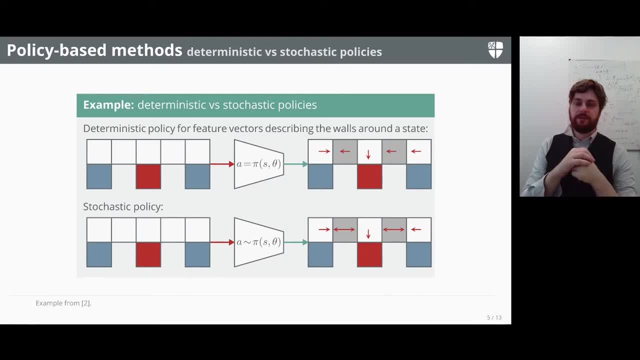 especially if you can't see your score. you can be in some room and this nightmarish monster might appear, but the room looks the same as another room, which is very safe room, where there's a massive treasure box just next to it. ok, so basically, in these kind of cases, policy based methods can be much better. 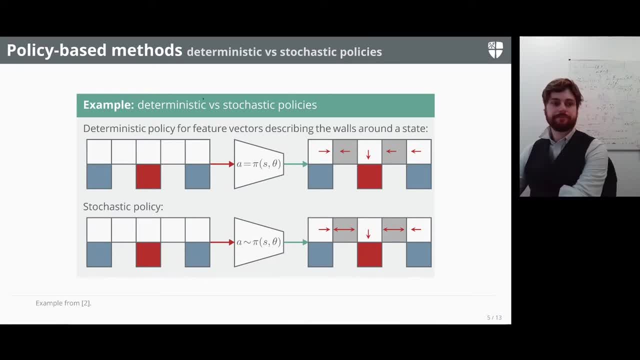 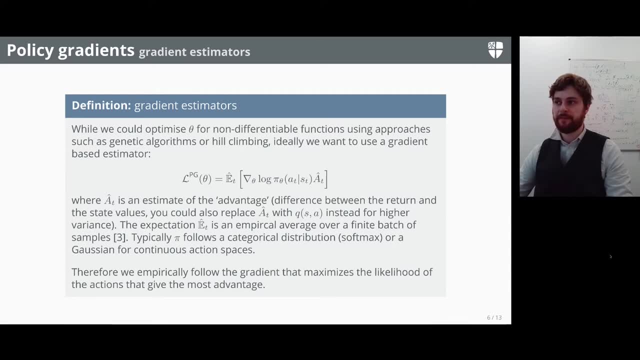 than value based methods like we've been doing previously. ok, so we said we're going to use a function, approximately 22 estimate policy, and we can actually use any kind of any kind of optimization approach for finding the parameters of this. So, if you have done the AI, 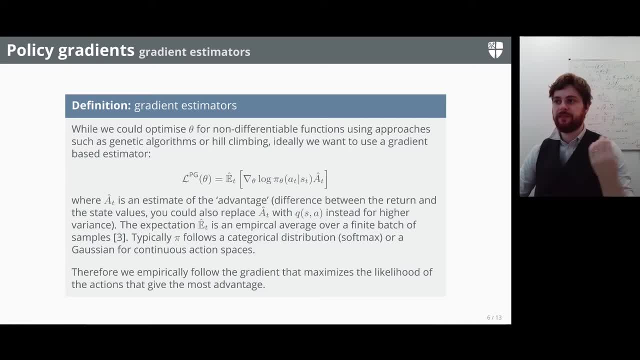 search module. you've seen how you can optimize functions using things like hill climbing or genetic algorithms, But what we really want to do is we want to use gradient-based optimization strategies. So with gradient-based approaches, we can parameterize our policy function using 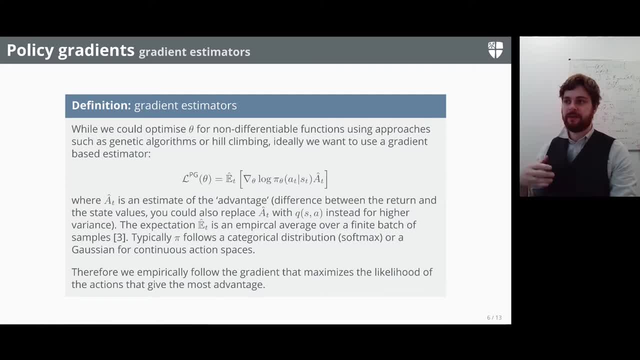 say, a very, very large deep neural network, and we can then take advantage of very efficient gradient updates. So we need to somehow come up with some estimate of the gradient and to do this we need to typically do some kind of empirical averaging. 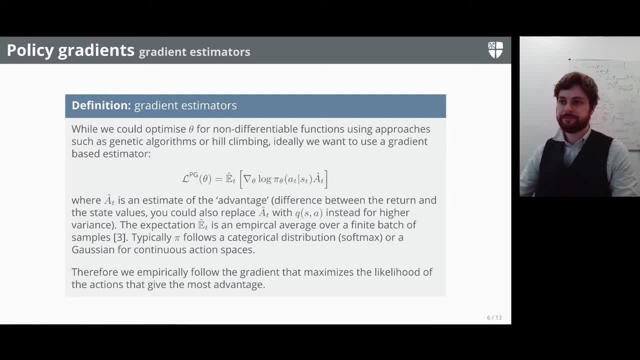 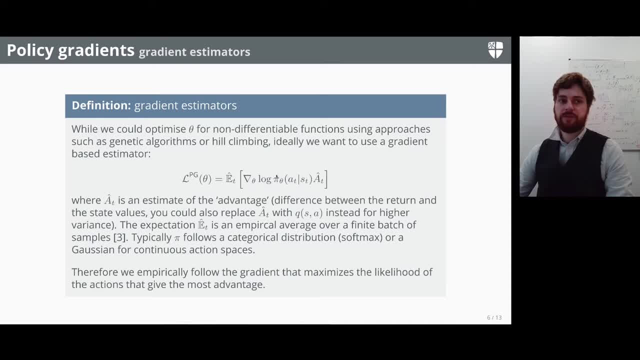 a log here And remember: this is a distribution over actions, This is a probability distribution over all of our potential actions. So, hopefully, the equation that's jumping out to you, how do we optimize the distribution? Well, we want to maximize the likelihood of that distribution. 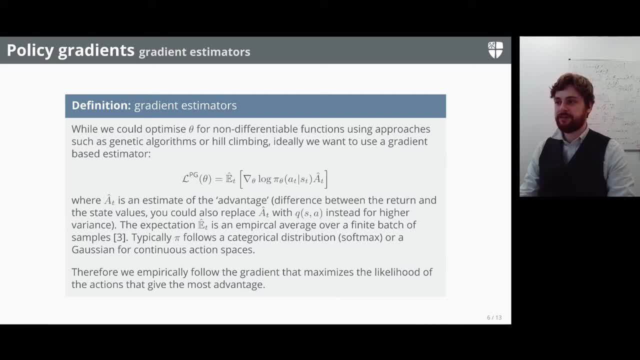 over the observations. So we want the max likelihood equations And you might be able to see this how that falls into the picture of the max likelihood equations. But try to think of this distribution as something we can have like. we can choose a distribution which. 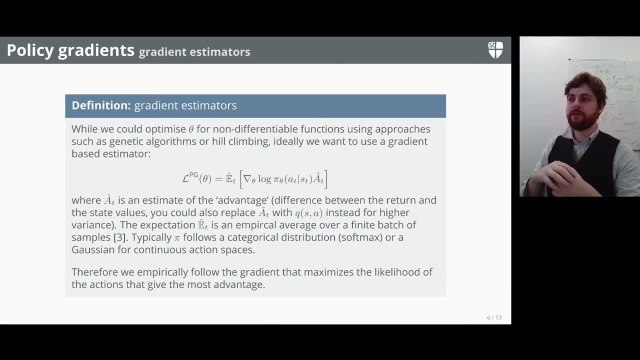 fits the kind of environment we're trying to do reinforcement learning on. So if you've got a discrete action space, like in Gravatar, where you've got a set of actions you can take, then we would want to have a categorical distribution, So like a one-hot encoding. 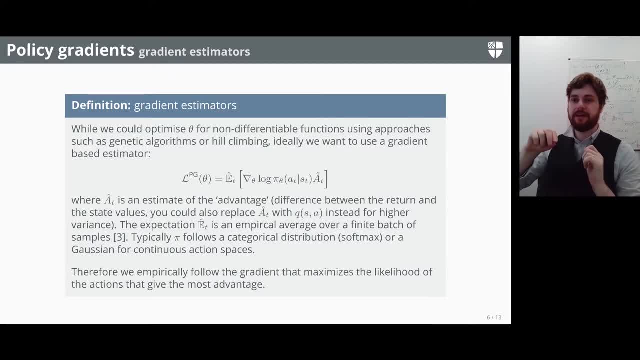 where the probability is one at the action we wish to take And to capture that you might want to use like a softmax function. If you recall from the energy-based learning, the energy models lecture, a softmax is just where you take your output of your neural network, you feed it into a softmax. 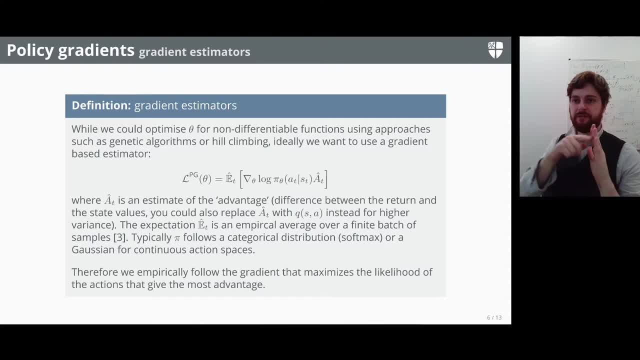 function and that ensures that the output, no matter what it is, always integrates to one and that it's non-negative. And it uses some exponentials in the numerator and the denominator to push the highest value towards one and all of the other values it pushes towards zero. 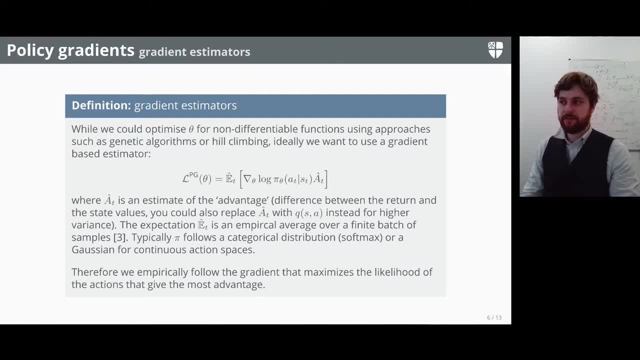 Or the most likely value it pushes towards zero. But you can also use like a Gaussian distribution. So if you've got a continuous action space, you might want to learn a Gaussian over the values of the action that you want. But again, we need the gradient of this distribution. 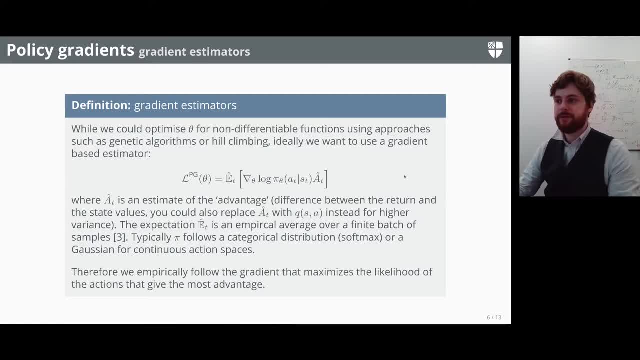 So we want the gradient of this function with respect to the parameters, so we can then optimize the parameters to maximize the likelihood. And if you remember the generative models lecture where we introduced the max-likely-acquired equation, if you remember the actual definition of the max-likely-acquired equation, 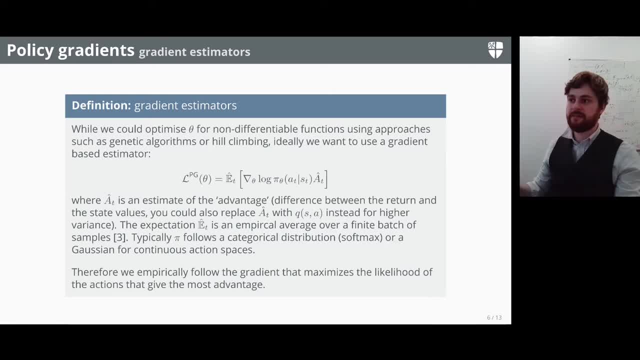 it had that big product in there, And then we could take the log of both sides and turn that product into an expectation which doesn't change the argmax of it, which is basically what we've done here, which is where the logs come from. Okay, so the last part of the equation here. 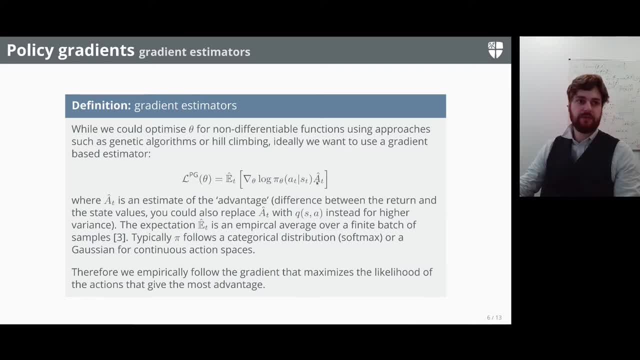 is particularly important. This is like maybe something new to what you're seeing. It's basically weighting the probabilities by whatever this value is, because we're multiplying the probabilities of this distribution by whatever this thing is. So this is really how we weight the distribution, And this- a hat here- is called the advantage function. 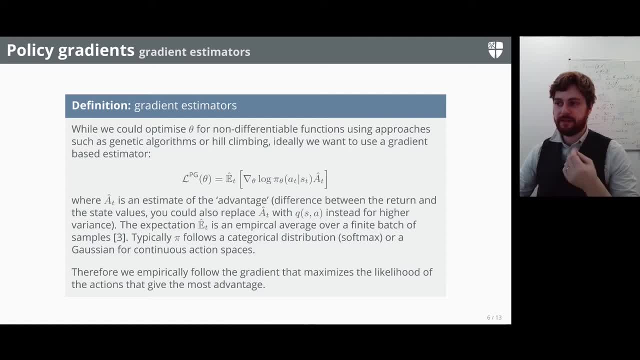 And it's just kind of like a more general form of the action value function with some nice characteristics. So the advantage by its definition is simply the difference between- yes, it's simply the difference between the return values and the actual values. So it's basically the same as. 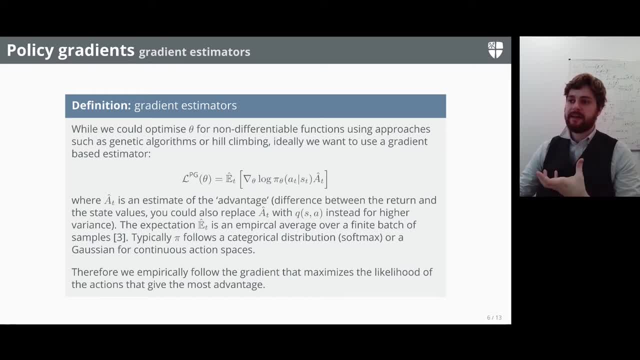 the action value function, but instead of telling us the value, it tells us the advantage to be gained. So because of that expectation, you can calculate it just by subtracting the value function from q And you can alternatively just replace that directly with the action value function. So you could just replace that with q. 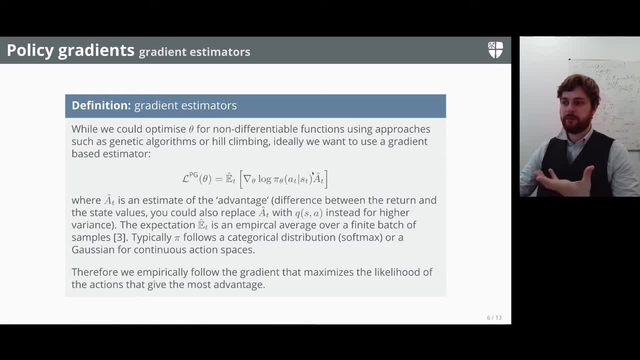 but this is just a little bit nicer to do this. but it would work to replace it with q. So the difference here is that using the advantage function as a equals the q value minus the value function. basically it has lower variance by taking the 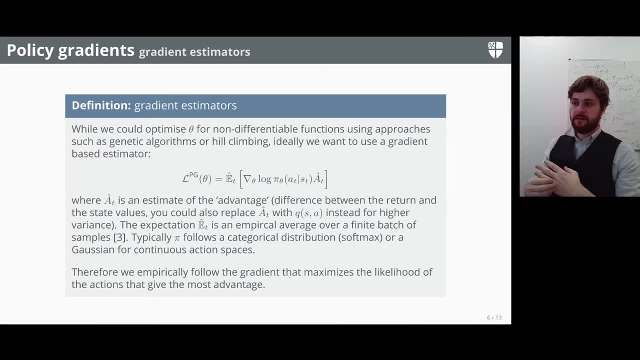 state action value off from the baseline. So we compute the returns by summing up our discounted rewards into the future and then we subtract that by our current estimate of the value function from our model. All right, so conceptually, what is this doing? And it's saying? I'll say it slightly: we defined a gradient of our policy. 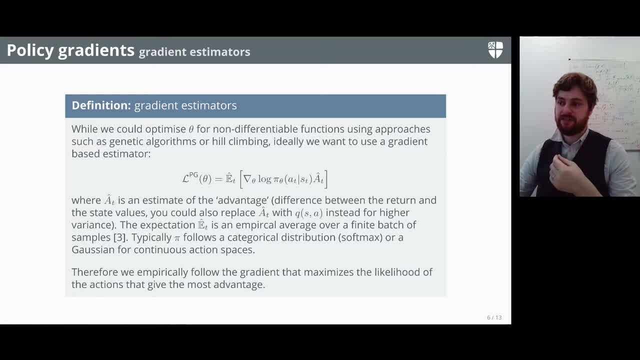 network, such as to maximize the likelihood of the actions that give the most advantage. So that's really what this whole equation is saying. So I'll say that again. We defined a gradient of our policy network, such as to maximize the likelihood of the actions or over the actions. 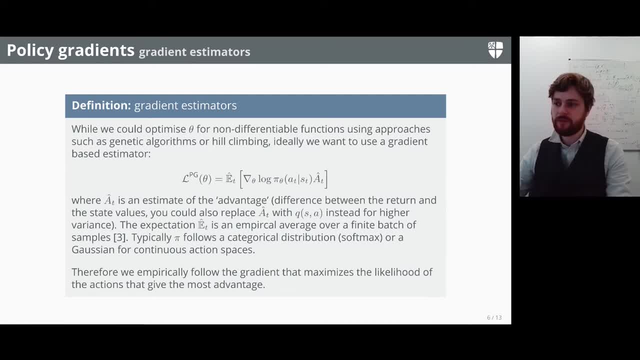 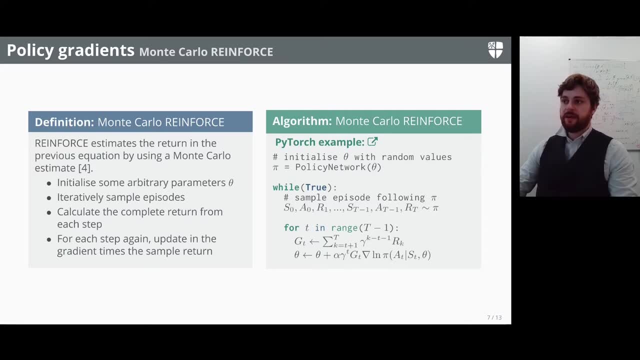 in such a way that gives the most advantage. So that's really what this whole equation is saying us: the most advantage, All right. so let's pull this all together now put it all together and kind of just naively implement it and see what happens. So for now, I want you to kind of just 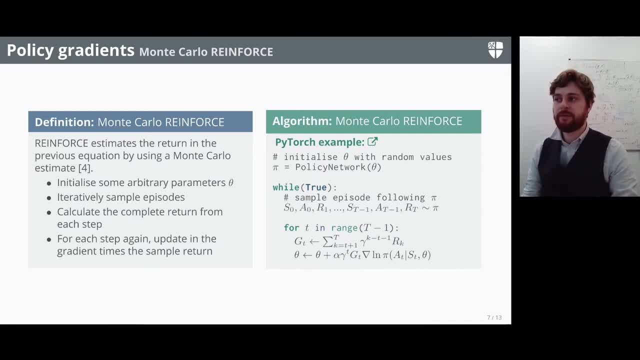 forget everything you've done with dynamic programming and Monte Carlo methods and TD learning and just forget, like, everything you've done with function approximators which introduces kind of stuff a little bit back again later. But we're just going to really naively implement a policy gradient based method by actually naively just manually computing the. 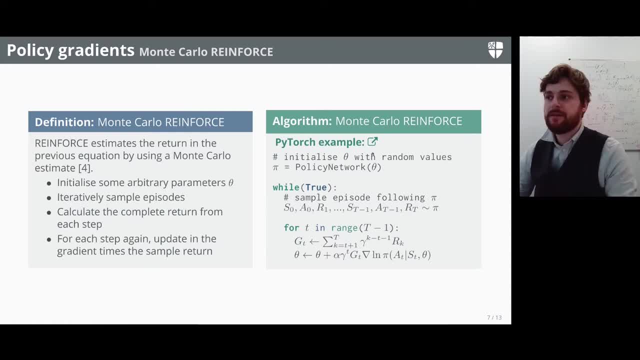 return And we get this algorithm here. So we're going to start by just initializing our parameters, theta, you know, initializing a random policy network with some random parameters, And we'll start by just sampling a complete episode here And remember, this is like a Monte Carlo method, So it requires complete episodes, all the 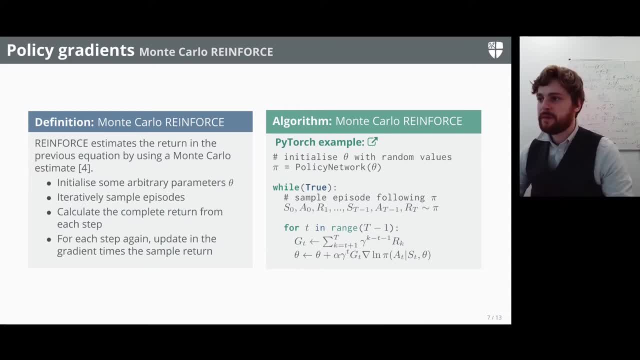 way into the future, complete trajectories, And then what we're going to do is we're going to just compute the return by summing all the discounted values by this discounted value function values of the reward going into the of that episode, And then we need to go, once we've 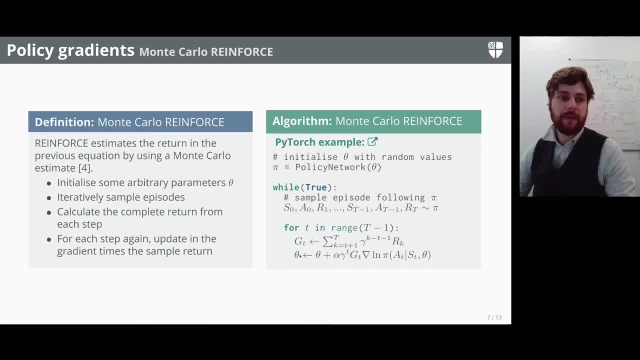 done that. once we've got this return here, we're going to go back through all of the states And we're going to update all our parameters, theta, by moving them just a little bit in the direction of the gradient that maximizes the log probabilities multiplied by. 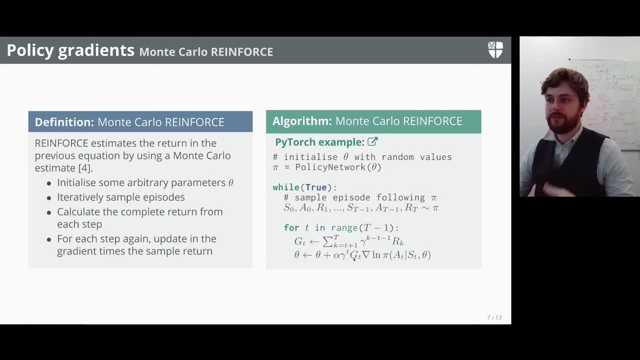 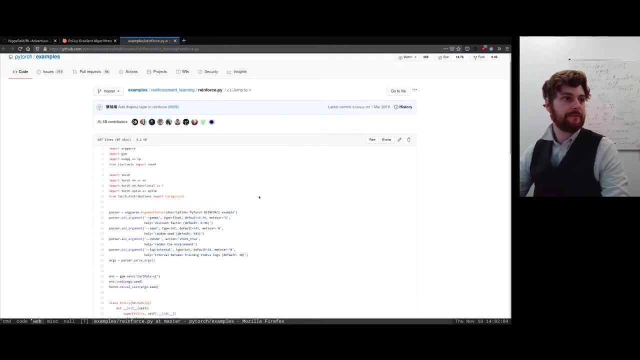 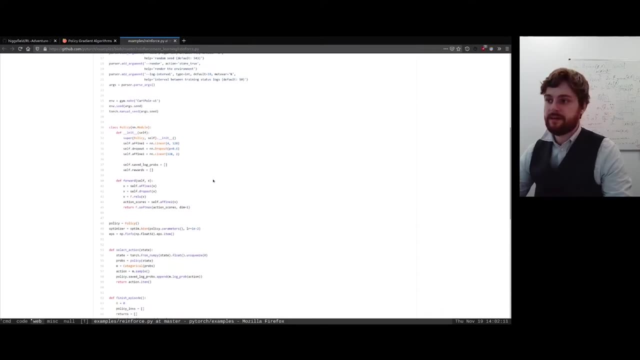 the return here that we got from that point onwards. So I just opened this code here. Okay, So here's some code from the reinforce algorithm. So at the top we have our policy network here. This is pi, if you like, in that code and this receives input states. 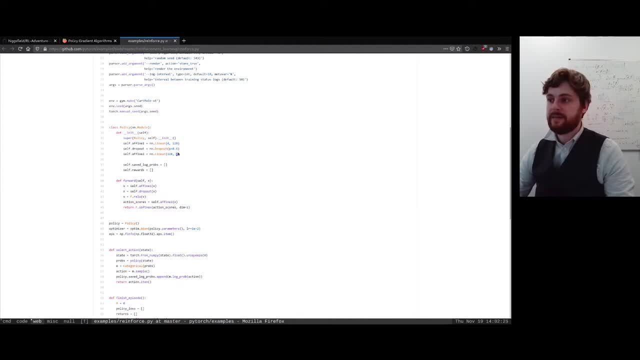 So it receives input states and outputs the action probabilities, Okay, and it does like a softmax over the actions here which turns that into a bit what turns into a distribution, And it makes it integrate to one by some exponential factor And then in this select action function, just here, 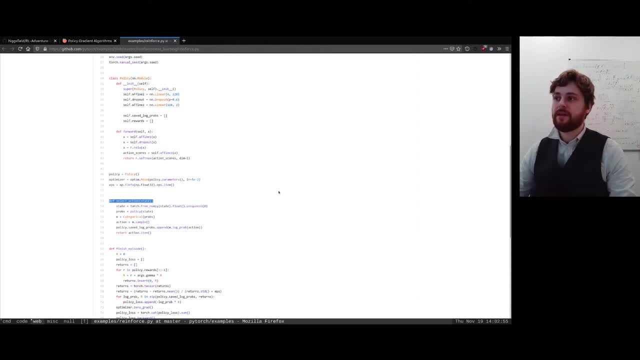 in this select action function we sample episodes. we start, we basically select actions by sampling from a categorical distribution, And that's what this code here does. So it samples from that, like softmax distribution samples an action from it, And also alternatively. 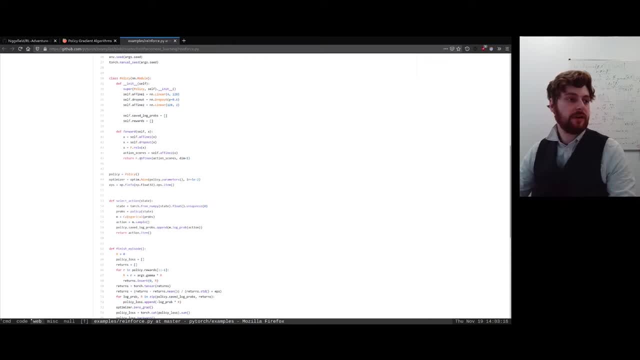 you could in PyTorch define this as a categorical distribution. you'd have to not use the softmax here and do things a little bit differently, But you could use a Gaussian here, for example. Then, if we go down to the main code at the bottom here: 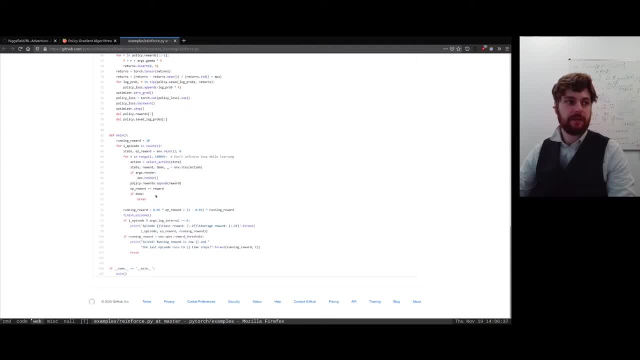 we basically start by sampling a complete episode. So just this whole code just basically keeps samplings. So this whole code just basically keeps samplings. So this whole code just basically keeps samplings- States, actions and rewards- until we're done And we aggregate or we push all of those. 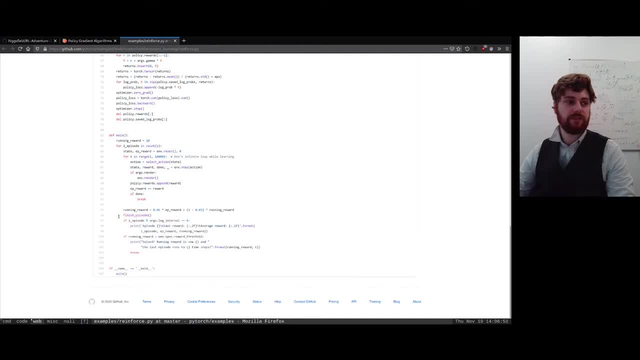 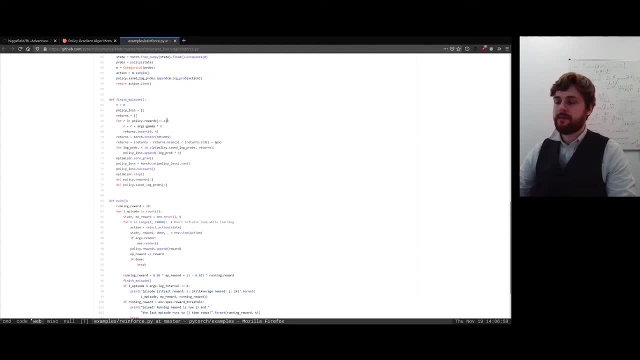 push all of that in And then it causes this finish episode function. So at this point in time we've got this complete episode in memory all in here And we basically accumulate our rewards at each state And then, when we sample the complete 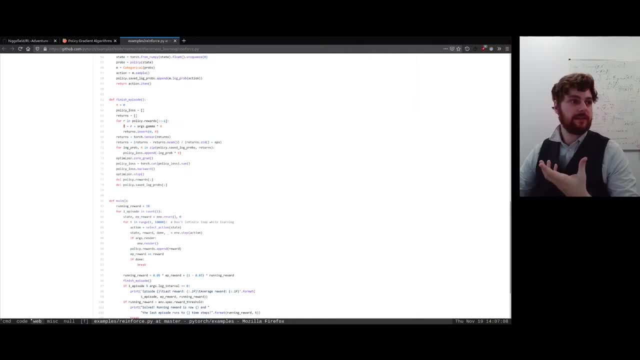 episode. we compute the return by this discounted factor here. So we compute the return going through And then at the end here we compute the loss, which is the log probabilities times the return, And then we backpropagate, updating all the parameters such as to minimize this. 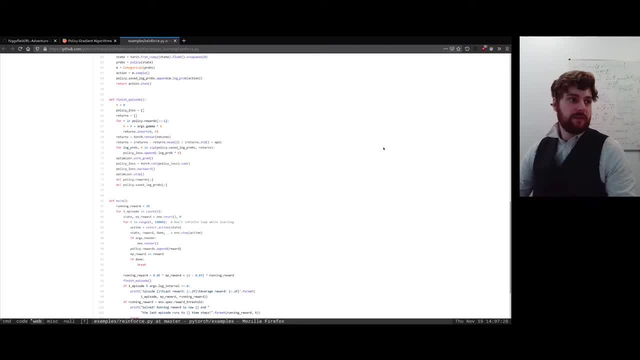 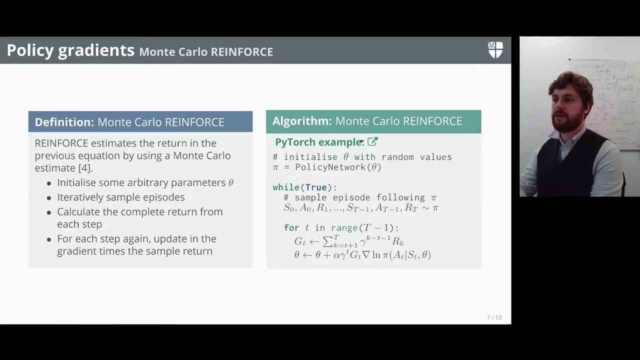 policy gradient loss here, Okay, And that's where we lost by the probabilities through by the reward. So this reinforced approach is really quite old now. It's an old policy gradient approach from 1988, and I wouldn't really recommend it. 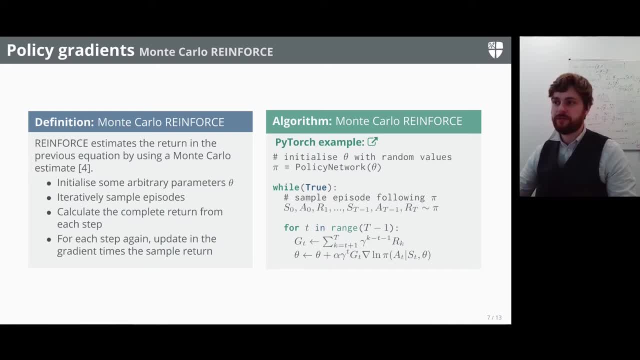 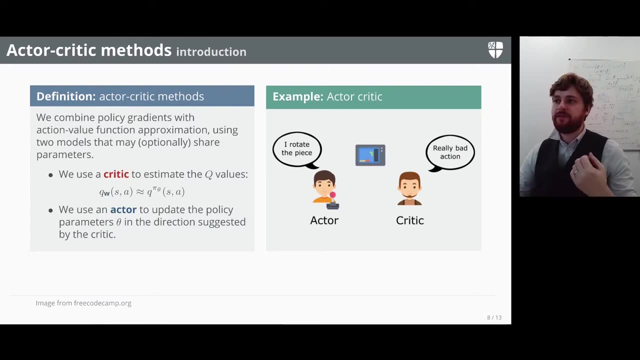 It's not particularly scalable and it requires this traditional approach for estimating the value function, But still it's a nice idea to just see how it can be done standalone and it works in its own way. So just a brief recap of what's happened so far. 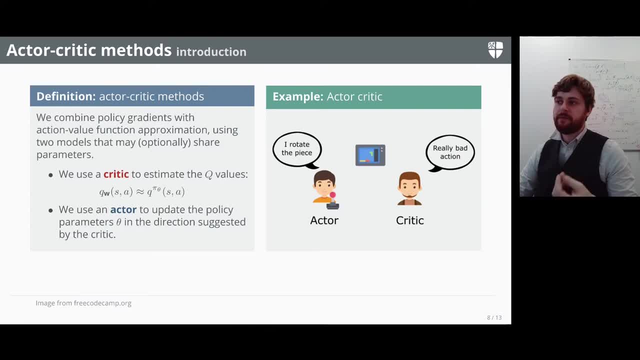 We've estimated the gradient of the return by taking a sample of our episode, but this gives very high variance. For example, if you're playing Atari, like Gravatar, it might be good that you get a good score sometimes, but 90% of the time you're going to get no score at all. 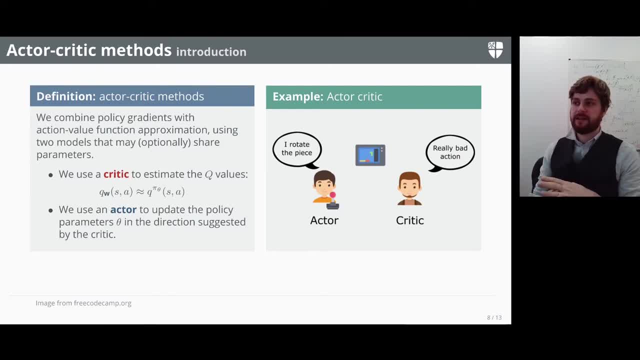 And maybe if you started running the coursework you're seeing this a lot. So you see that most of the time you just get 0, 0, 0, 0, 0, 0, 0, but occasionally you get quite a high score. 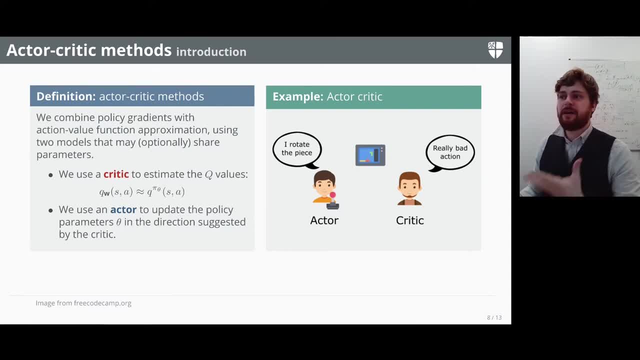 So you've got this high variance going on, And that just comes from the randomness of what happens. Maybe most of the time your ship just gets dragged into the killing star at the beginning of the game. So you get this very noisy play. 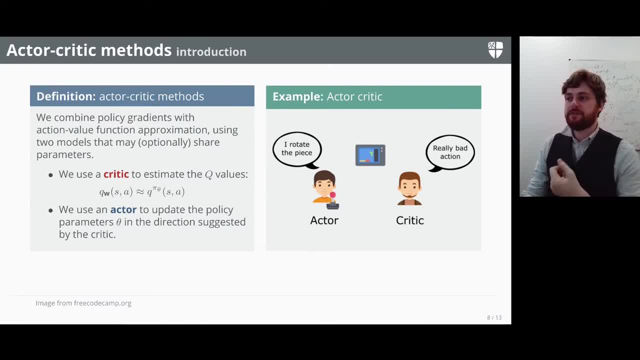 Now, the main idea of actor critic methods is that instead of using the return to estimate the action value function, we're going to instead use a critic function as an approximator for that estimate. So we're going to bring back the ideas from last lecture. 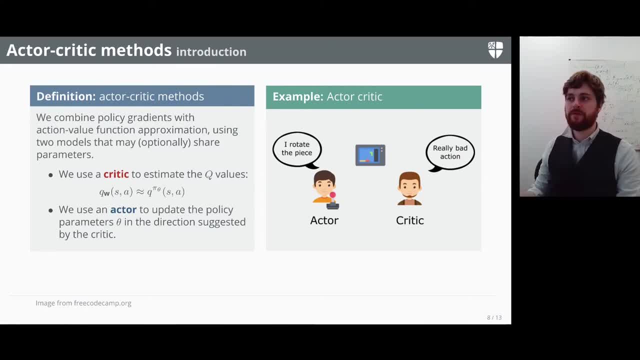 and we're going to combine the action value function approximation with these new policy methods. So, like last week, we'll have our true action value function, which we're going to estimate using a function approximator, But then we're going to use that just as a component. 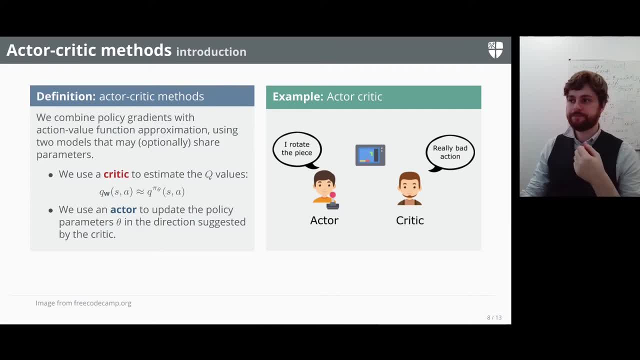 for our policy gradient approach as a substitute for q, pi, And this means that we have now two models with two sets of parameters, which is why they're called actor critic. So you have this critic which judges the actions, like the example here, where we have an actor which 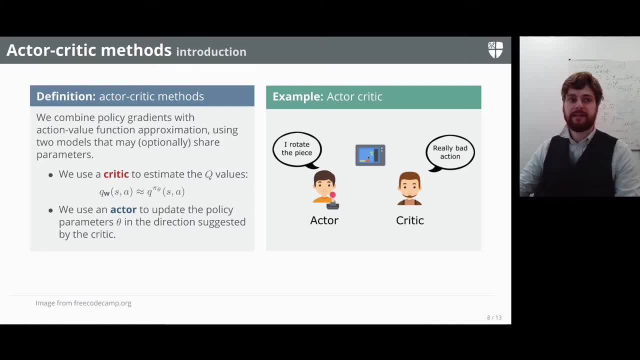 chooses an action. So this actor here they're playing this game of Tetris and it chooses the action. It's trying to say: is it good for me to rotate this piece? As one of its actions, it could press left or right. 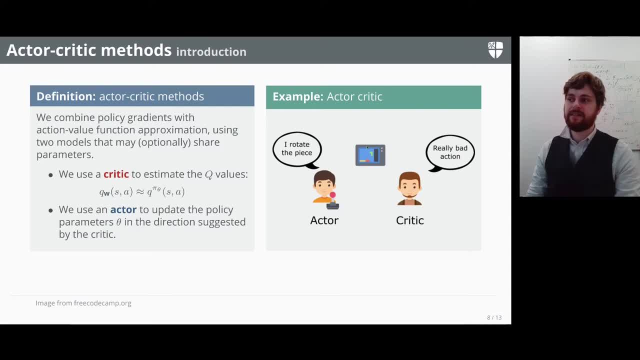 on the keypad to rotate the piece in a different way. And the actor thinks it's a good idea to rotate the piece, But then the critic says no, that's a terrible idea to do that. And the critic says rotating that piece. 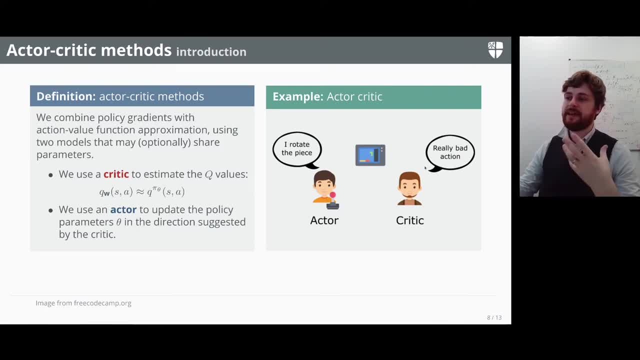 is a really bad idea. So, in other words, the actor is responsible for taking actions or acting and it makes all the decisions And the critic is just there to, As a sort of spectator which watches the actor and what it's doing and evaluates. 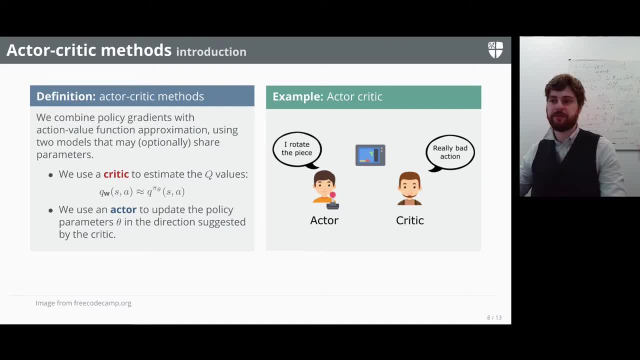 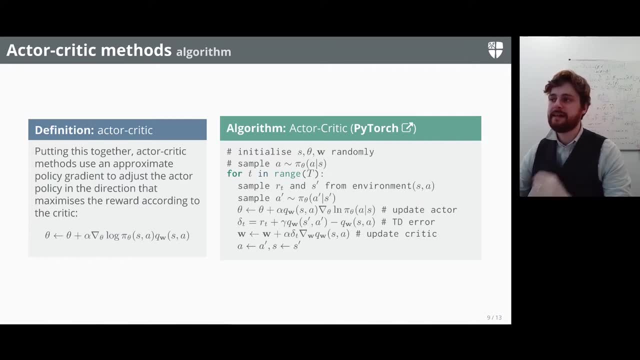 whether it thinks that's a good or a bad thing. They kind of bootstrap from each other. OK, so, putting this all together, we're going to combine the actor and the critique into a more formal definition of the actor, critic approach and the algorithm here. 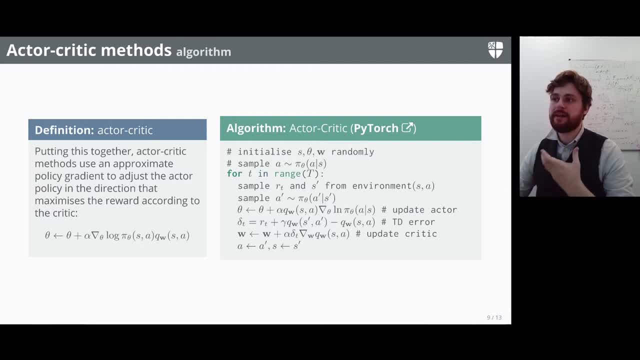 So we're going to use an approximate policy gradient to adjust the actor policy in the direction that maximizes the reward According to some critique function. So if we look at the equation down here, we see that the critique or Q, with the parameters W, just estimates the action value. 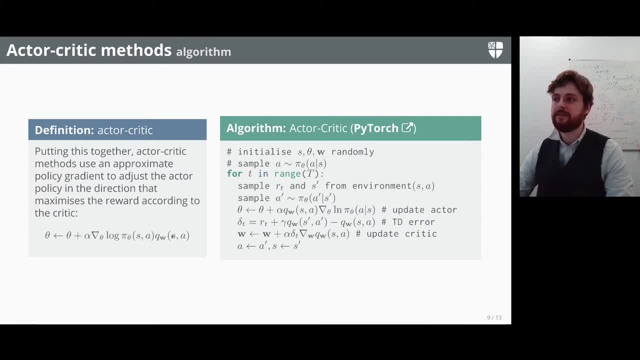 function given some state in action, repair estimates, the value function, which tells us basically how good the reward is or the direction of the reward is at. And then this other bit here is just the same as before. So if you remember, we could also have the advantage here. 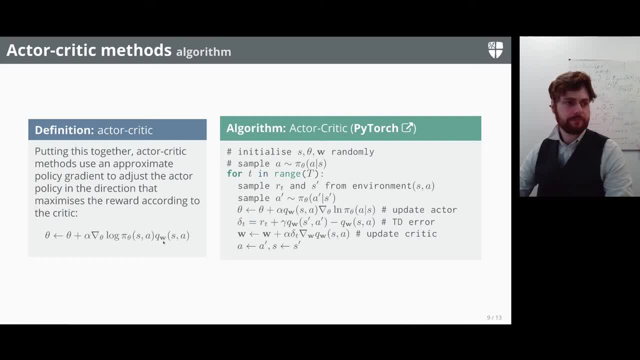 So we can have an estimate of the advantage. So we can have an estimate of the advantage here. So we can have an estimate of the advantage here. So we can have an estimate of the advantage here, advantage which would be equally valid. But basically, we just update the parameters. a. 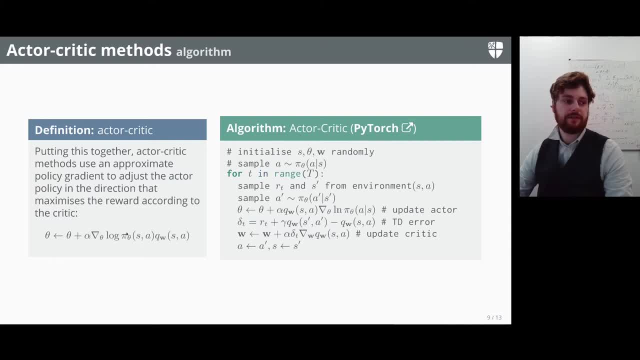 little bit in the direction of the gradient that maximizes the likelihood times, the advantage or times the. in this case we have this q-network here, this approximator, here parameterized by w, And this policy network is parameterized by theta. So this is just like wrapping it. 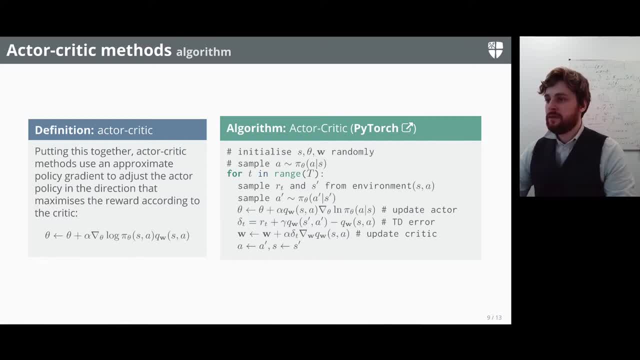 all together now. So the critique, this qw here, says I think this action is good in this state, or it says I think this action is a bad idea to take in this state. So we're going to update our parameters, theta, a little bit in the direction of the things that the critique. 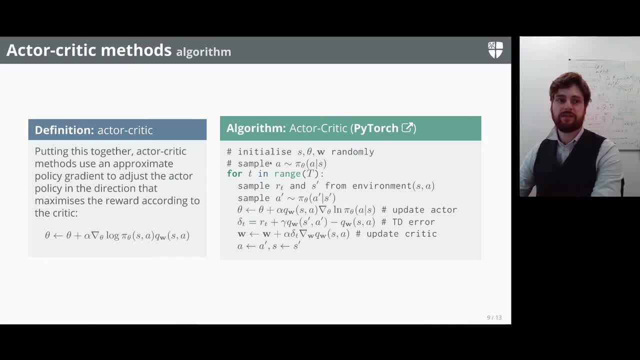 says are good, All right, so let's just go through this algorithm now. So we start by just initializing our state, Okay, Okay, And we randomly initialize our deep neural network parameters and the weights, also the parameters of the critique, And then what we do is we sample an action from our policy. 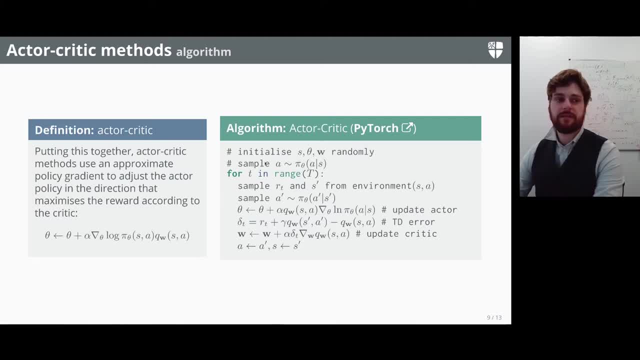 So from the actor network I should say so this is sampling from the actor, conditional one being in this state here It tells us how good it is to take action, And initially that's obviously just random. So it's almost like a random action. And then the actor network. 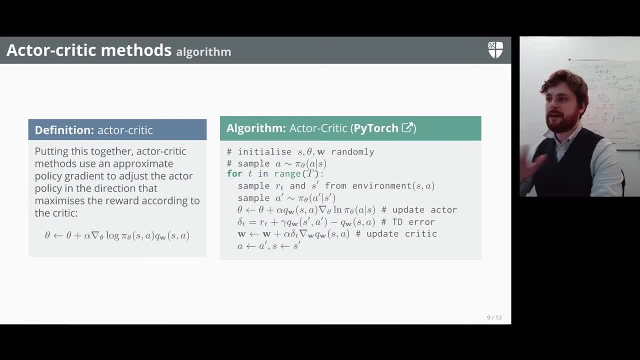 does a softmax function over its output neurons, which gives us a set of probabilities which we can actually sample from that categorical that we see in pytorch. Then for t time steps, here we sample the reward at the next state from the environment, conditional on taking. 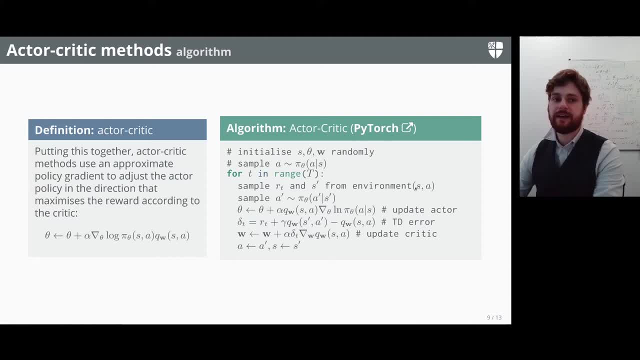 that state conditional on taking that action at our current state here, And if you're playing Atari, this just basically takes you to the next state, which is the one we're going to state s prime when you take an action, For example if you press the fire button on your controller, 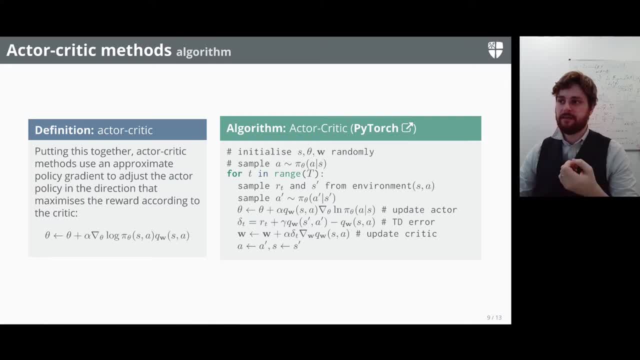 it tells you the reward you're going to get at time step rt, the reward you get at r, subscript t, And with that information you can then sample your next action from the actor again And you basically feed the actor network with the new state that you're in. 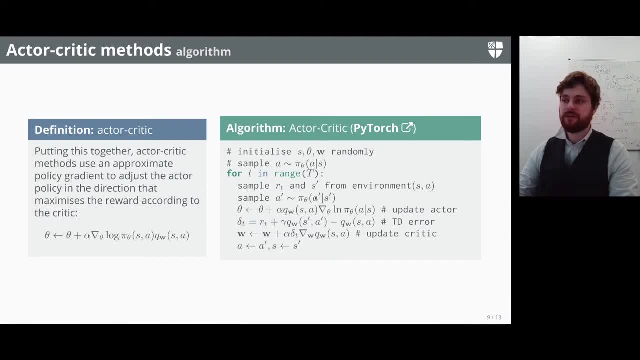 and that gives you the distribution over the next actions that you're in, And that's how you do that kind of look ahead. Okay, and now what you do is you update your actor as per the equation. So basically, you optimize the actor network parameters in the direction that maximizes the reward from the critique. 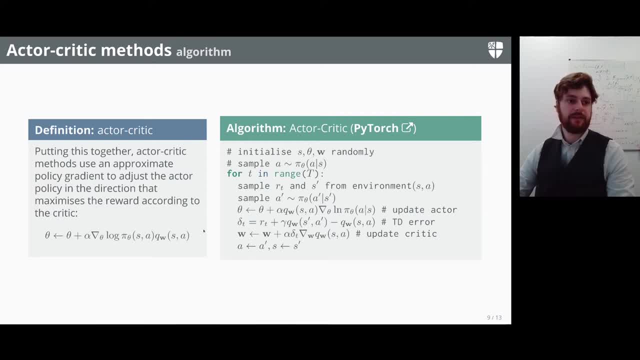 here, And this is just basically the same as that, although these things are swapped, All right, and after we've done that, we update the distribution over the next actions that you're in, So we can now update the critique in the same way as the last lecture, but using TD learning. 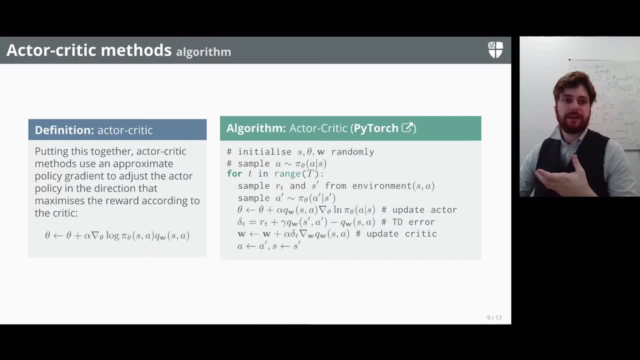 So we compute the TD error, which was the immediate reward plus the discounted value of being in the next state, Okay, the discounted value of the next reward minus the current reward, which was basically our Bellman equation. And now we can use that to: 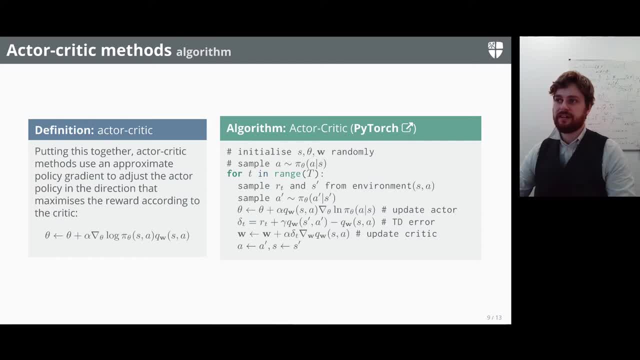 update the critique network weights w, just like in the last lecture, to estimate this action value function. So we update w a little bit in the direction of this gradient And note there's like this, learning rate alpha here. there's two alphas here. Actually it's quite common to have different alphas. 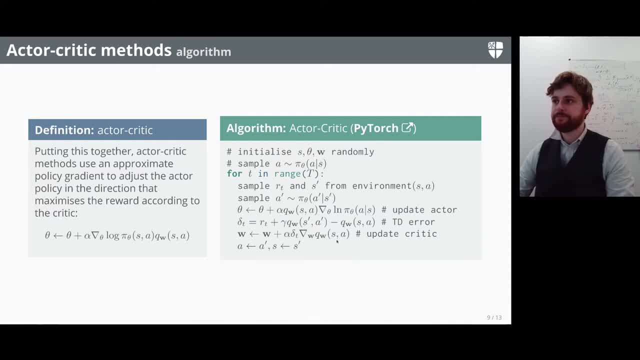 for the actor updates and for the critique updates here. So you can have like alpha subscript one and alpha subscript two. but I haven't really shown it in this algorithm here. But it's quite good to just tune those different learning rate parameters between the different actor and critique networks separately. 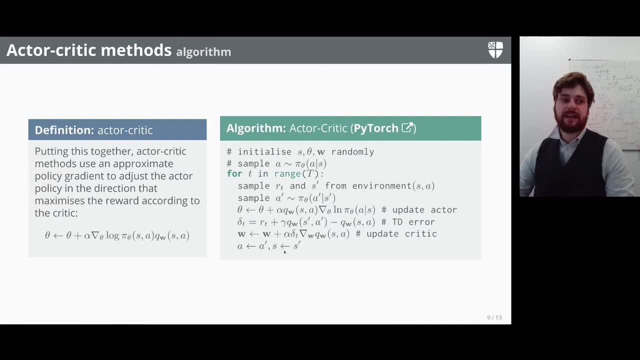 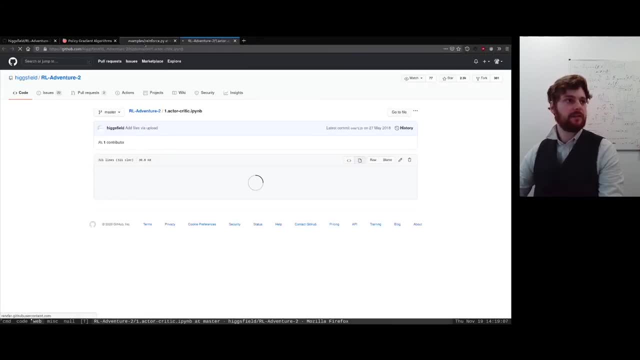 So, lastly, we can basically update our state and action to the next state and the next action, So we're set up again correctly for the next iteration. So with that all in place, let's just have a look at some code to do this. 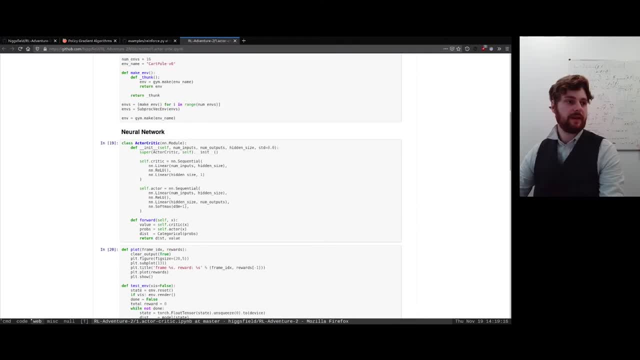 Okay, so this is all just the standard thing again, but this time we have two networks. We have our actor network and our critique network, And both of them receive states- just the number of states- as input. so this is basically your observation of your environment. so it could be like your memory. 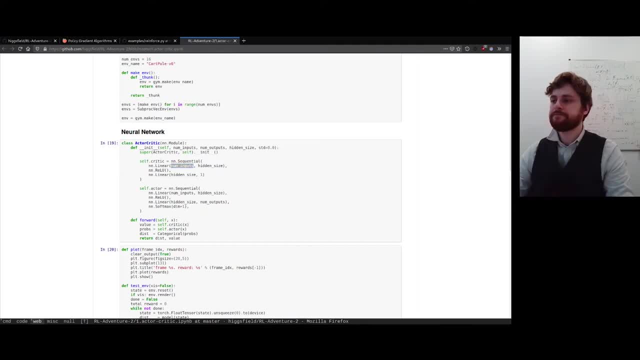 in gravatar or it could be like pixel values on a screen and the actor chooses like an action, so it has the number of outputs. so this is the number of actions we can take as our outputs and we do a softmax over those to turn them into distribution, whereas the 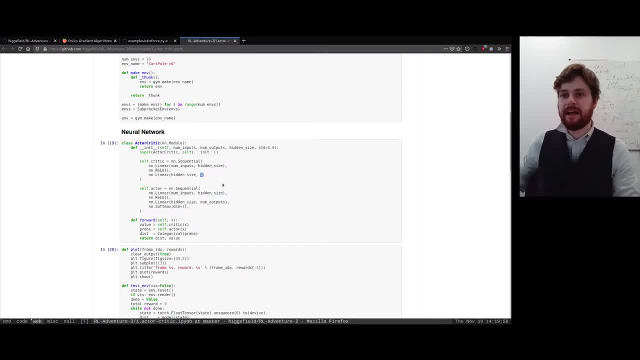 critique is just like a judge which says how good it is to take a particular action or not. so it's just got a single output neuron which corresponds to how well it does all right now in the forward pass here you see that both networks take as input the state. 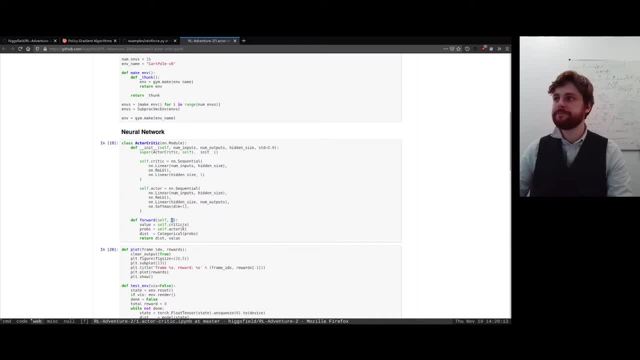 so you take this input state x and you pass that into both networks, but then the output distribution. here we wrap in some categorical which allows us to then later sample from it. this is a really nice helper function you get in pytorch which lets you sample from the underlying distribution. so it's quite nice. 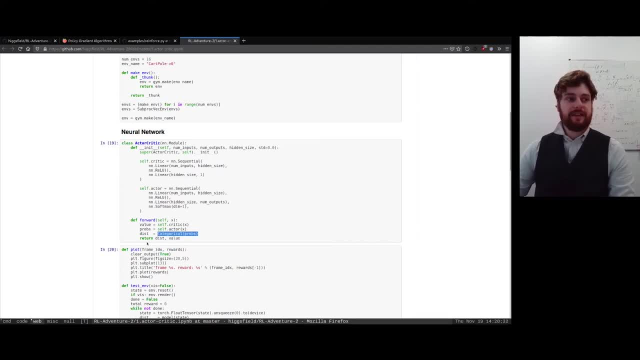 to use, so you can change this to like gaussian and sample from a gaussian as well if you want a continuous action space. so also the value of the critique is: is returned, as well as the distribution function, which contains the actual probabilities themselves. alongside that ability to that wrapper to sample from it, sample new actions from it. okay, um, and this code in: 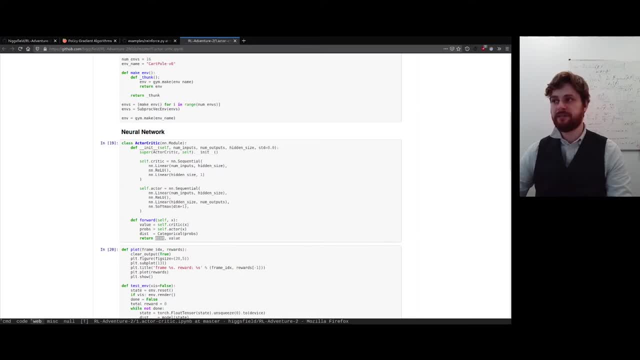 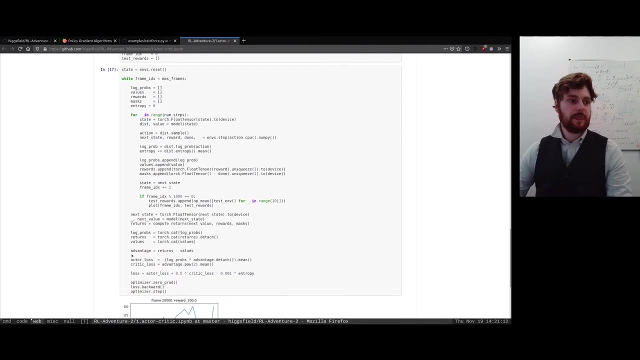 implementation extension, sorry, an extension of actor critique, which is the advantage actor critique which we covered in the very first equation. so instead of the q values it, it uses the advantage. um. so if i just scroll down a bit, so yeah, this is the advantage actor critique. so instead of just the q values, it does the actual advantage definition, like we saw in the first. 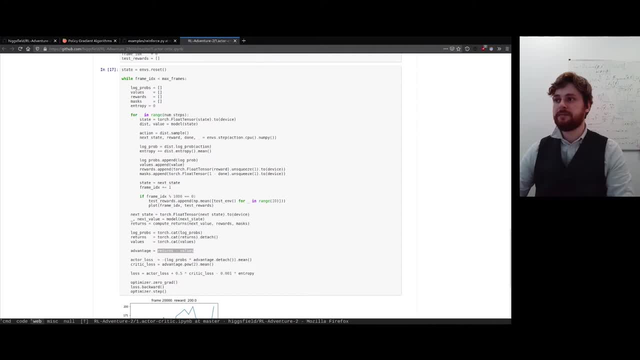 equation, so it's the returns minus the values instead of just the td error. here we train on the advantages, okay, um, but basically algorithm is otherwise really similar, which is that we start by um, where is it trying to find it? yeah, we start by just this, this dot sample, because remember the 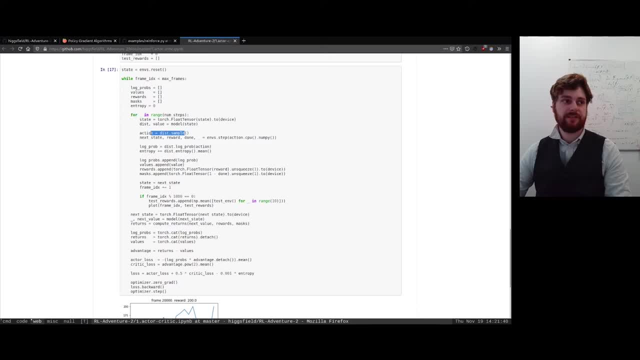 model returns the wrapper around the distribution so we can sample our actions from the actual underlying action distribution. and then we want to sample the next state and the reward from the environment under that uh action. okay, so this gives us the next state in the reward for taking that action within the environment. 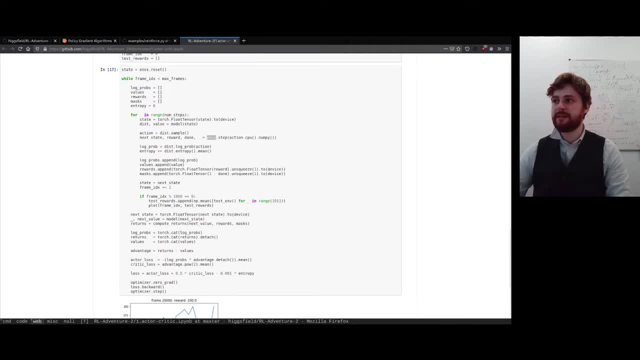 um, and then we take the log of the action probability to work out how likely that was okay. and there's like a slight addition here which you can read about in the a3c paper, which is that they add some kind of entropy regularizer, um. but this is basically this, something you can read about in 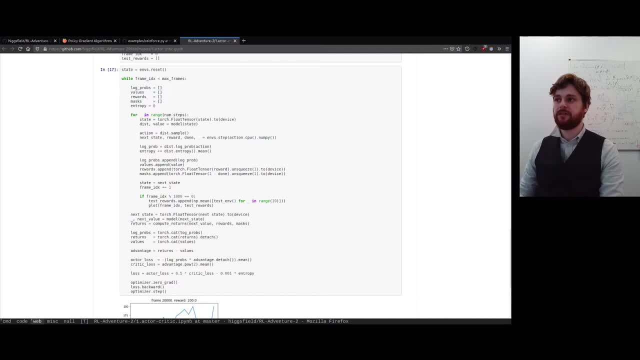 the paper and it encourages a little bit of extra exploration. so according to their paper, the entropy loss encourages more logarithmic contribution and it encourages more entropy, encourages more of a uniform sampling rather than just letting any one particular action dominate all the time. So that's just some nice little contribution of that paper. 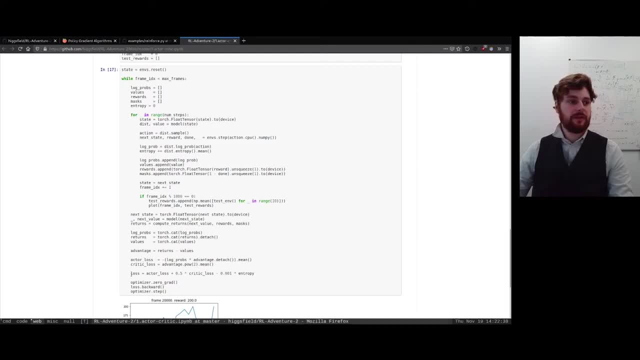 But lastly, at the bottom you get the final loss down here, which for the actor is just the log probability multiplied by the advantages we've seen. So it tries to maximize the likelihood of the actions that the critique thinks gives the high value. 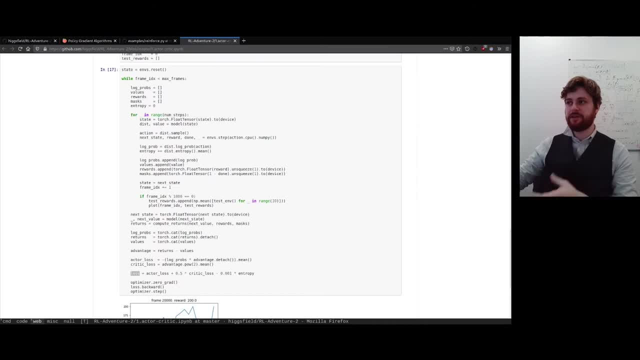 And note there's like a detach here as we don't really want to back propagate through the critique for this loss. But then we have the critique loss, which is simply the L2 norm of the advantage. So it tries to make the value function, estimate the. 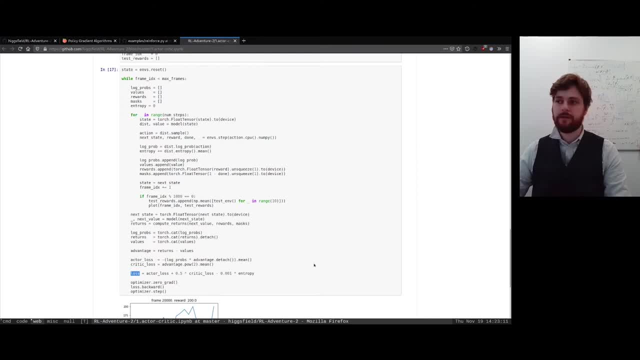 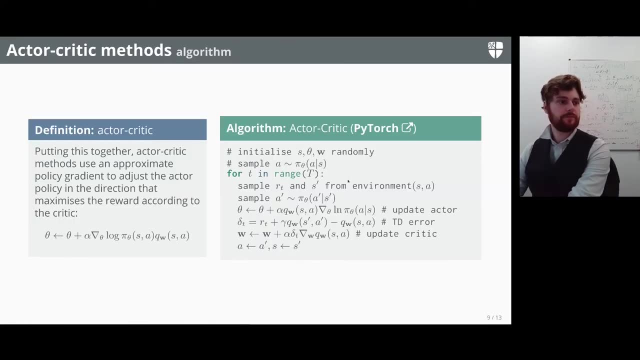 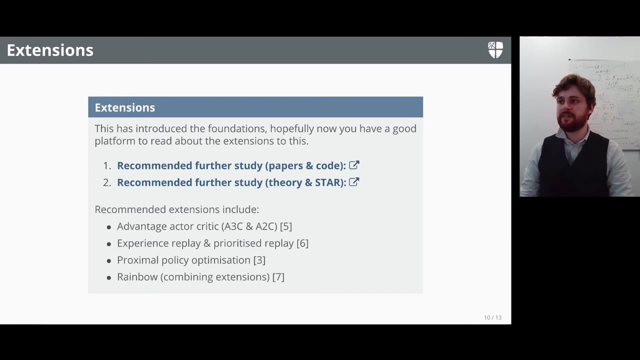 it tries to make it match the return, I should say, All right, That's kind of how that all comes together now, And I think that's really the foundations of what we've put down there. So in practice, there is quite a lot of extensions to this. 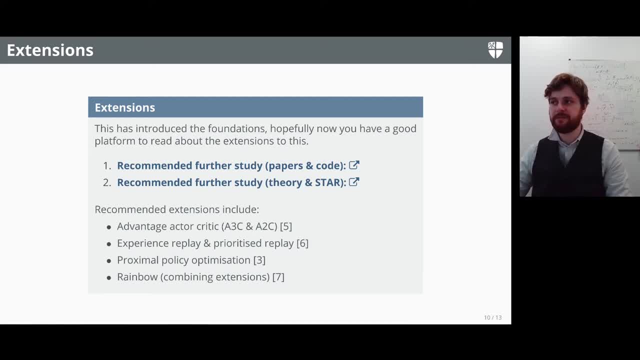 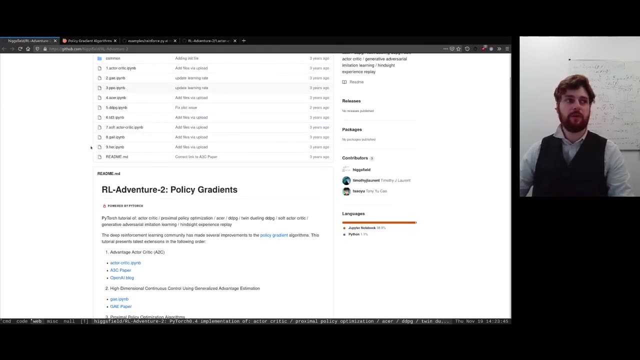 So I strongly recommend you spend like at least a couple of hours reading recent papers that build on these ideas. And in the top link here there's a nice set of papers in PyTorch implementations- we'll just open that now here- And these really introduce quite a lot more tricks. 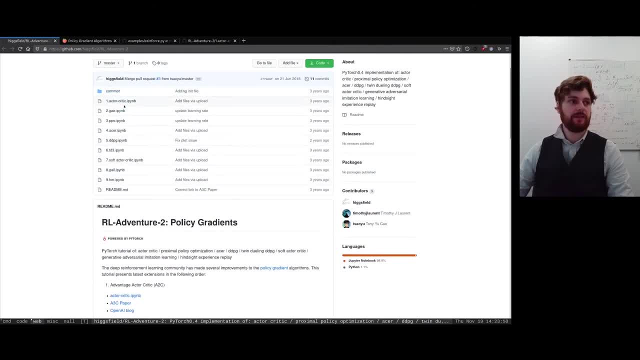 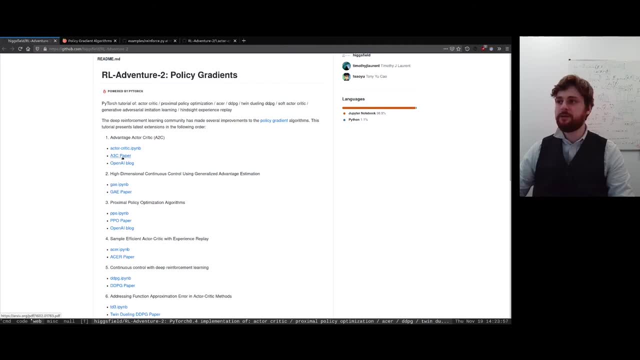 available to you. So I'd recommend just scanning through the code at the top here. So click through each of these and having a scan, and alongside the code here you also have the papers, And then again you can go into like one of those papers. 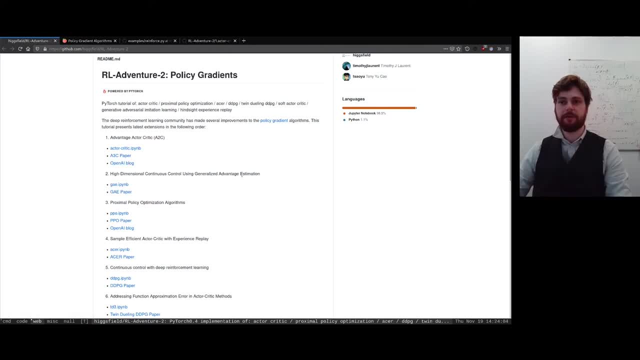 and just have a quick look through, pick up the concepts that you're familiar with now, with this foundational active critique knowledge, and just see how they extend the basic idea and what their contributions are. The second link here links to Lillian Wang's blog. 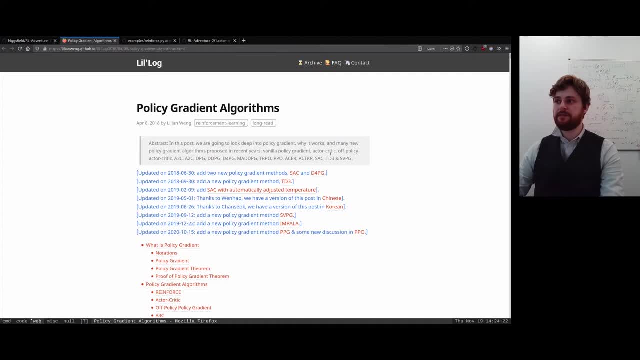 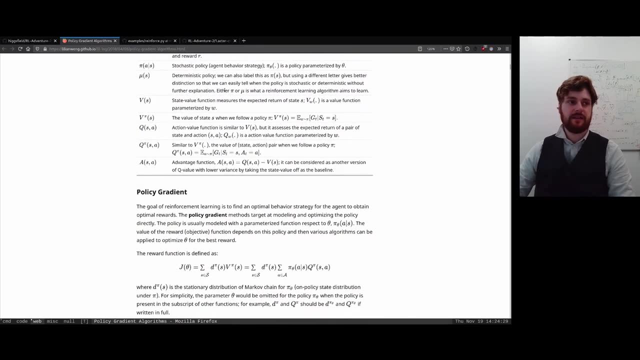 And this is a really nice little study. It's a really nice little study, It's a really nice little state-of-the-art report, or we call it a STAR, And it just kind of goes through very densely the kind of notation and theory. 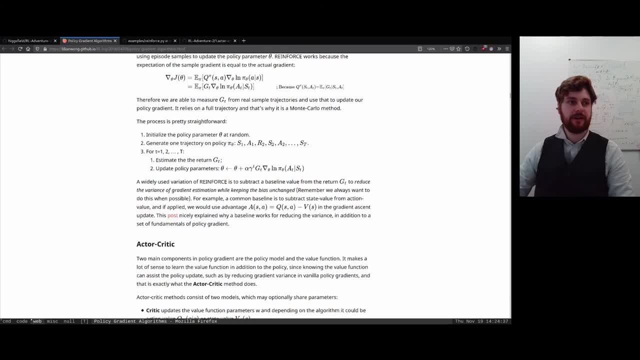 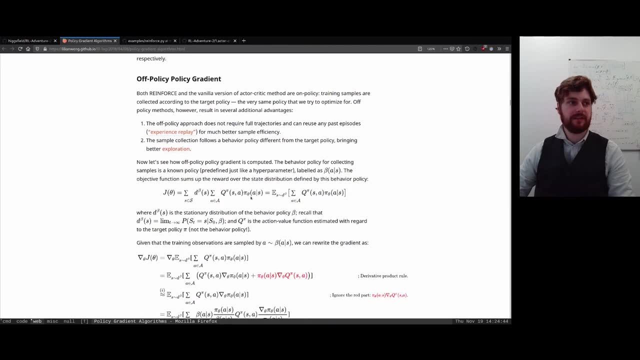 behind some of these techniques. So she just very quickly introduces very mathematically dense theory of reinforce active critique methods- the kind of similar algorithms that we've seen today- and goes through quickly into more state-of-the-art techniques- And there's just hundreds, I think, of them. 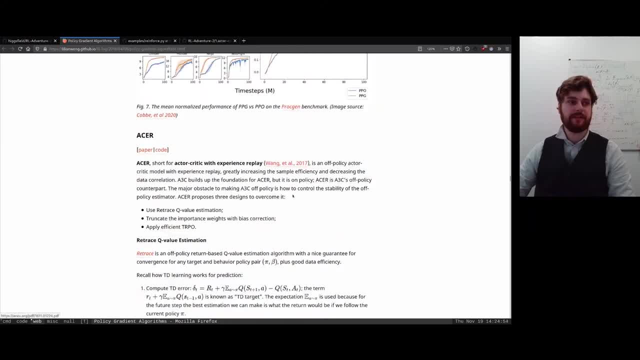 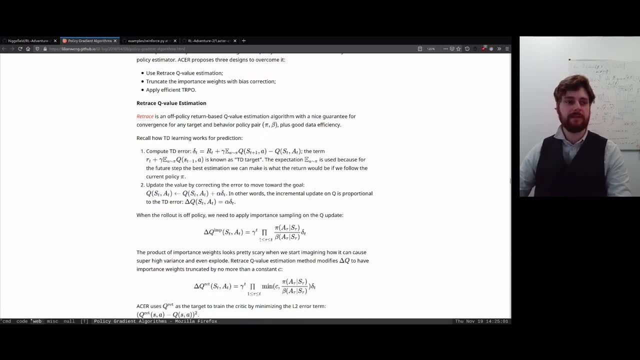 There's hundreds of these available And this covers quite comprehensively, but it's hard read. I'd recommend, rather than just trying to get everything from this blog post, actually opening up some of the papers, maybe YouTubing, and seeing other people. 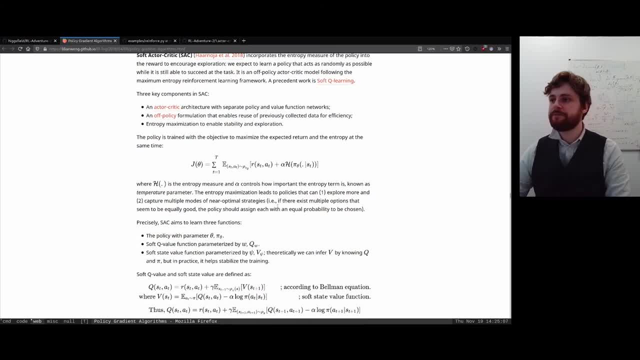 explain the concepts as part of learning. Yeah, do like look at the results in the papers, because a lot of the papers can be very, very mathematical and long and extensive, And then you look at the results for something like Atari and it turns out that it's worse. 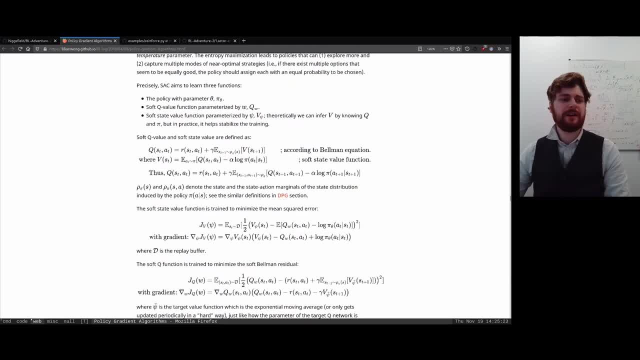 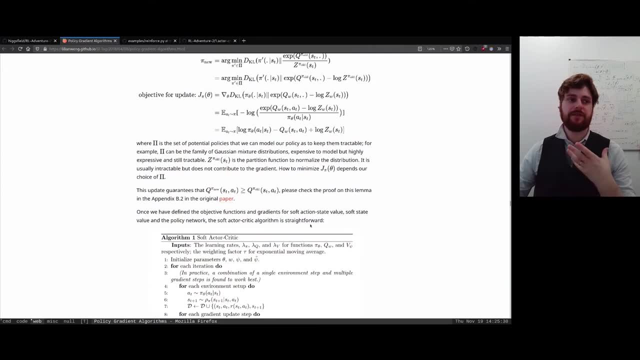 than just the naive baseline algorithm. This kind of stuff really is, I would say, almost first year PhD level, So it's quite advanced. but it is worth having a glance through to see if anything's relevant. We'll see if anything's useful. 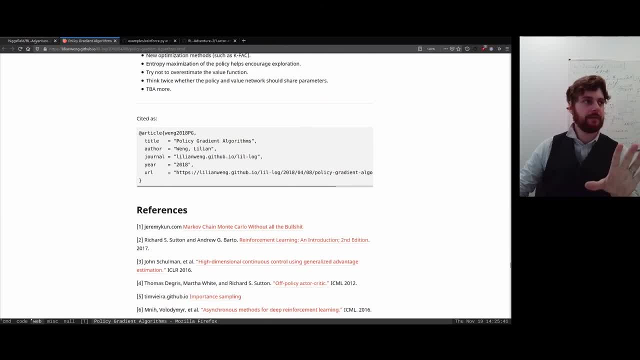 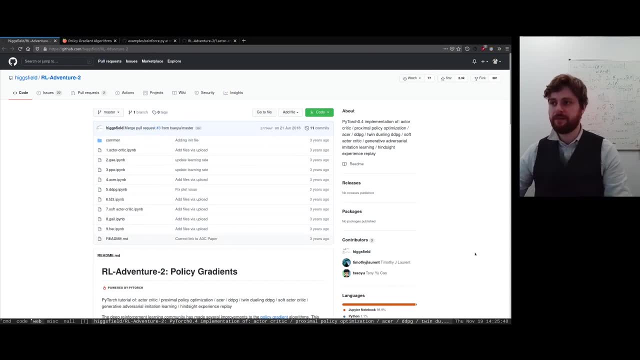 So don't be put off by this blog here. I would recommend starting with these kind of maybe looking at some of the extensions here as a good place to start if you're wanting to pursue these kinds of methods. So in addition to this I've picked out actually 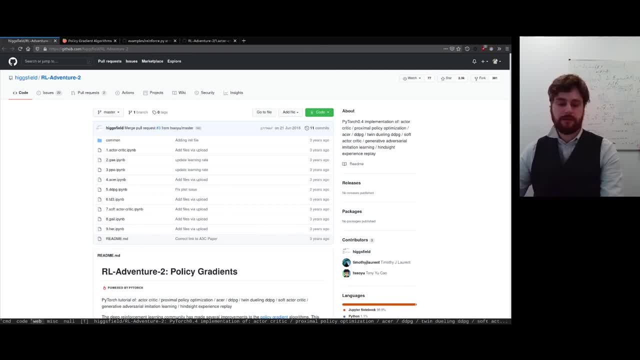 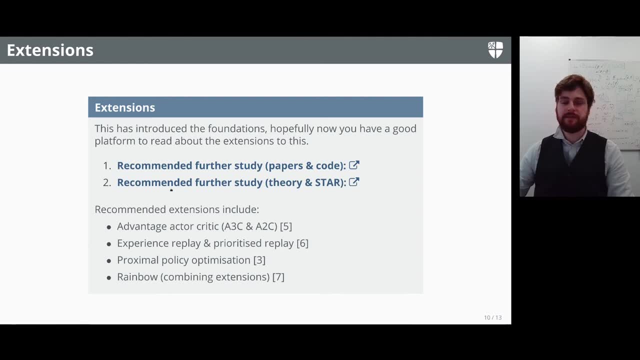 I've picked out some of the things that I think are really useful, Like the following. sorry, I've picked out here, to make your life a bit easier, four papers which I would recommend studying these in a little bit more detail. 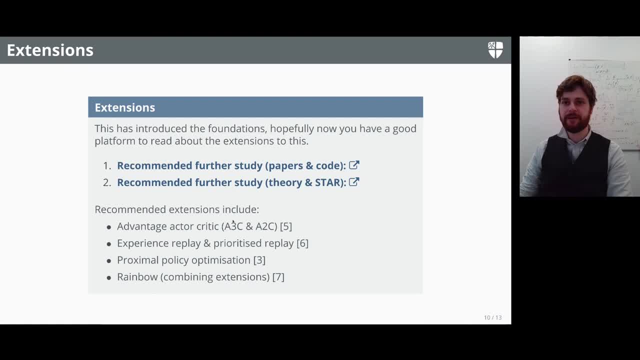 So, rather than just being overwhelmed by, say, Lilian Wang's blog, you might just want to study these for in a bit more detail. And when you study these papers, I recommend the Feynman Technique for Learning, which is basically where you 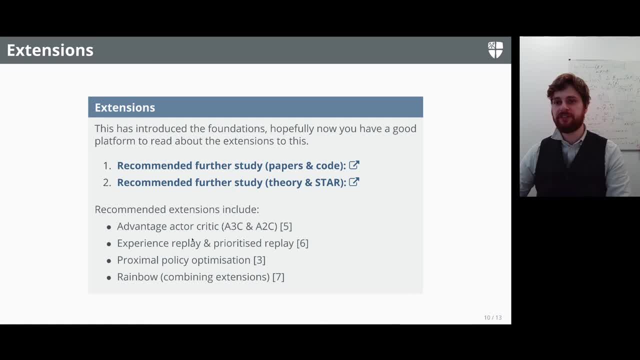 if there's something complex or difficult, or a word or a terminology or a piece of mathematical notation that you find really challenging, just write down whatever that is on a piece of paper. then go into Wikipedia, go onto YouTube and listen to people explain whatever that thing. 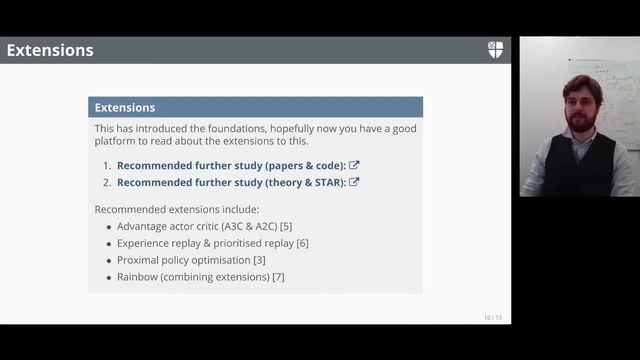 that you're stuck about is: Maybe it's some advanced piece of mathematics And then if, in the process of trying to explain it, like you were to say a child or someone, you can't do that, or there's another piece of mathematics. 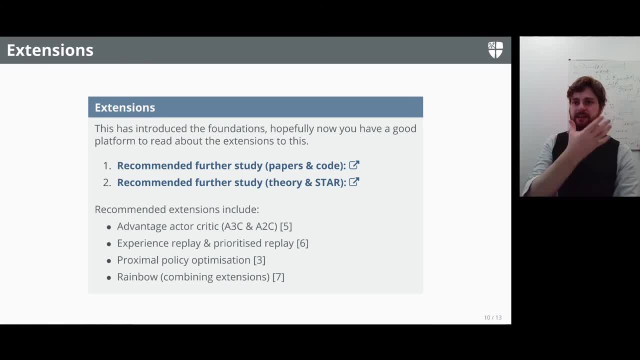 you don't understand in Wikipedia relating to that concept, then just create a new piece of paper with that new piece of mathematics, put it on the top and try and explain that concept to a child And basically that process creates a hierarchy of the gaps in your knowledge. 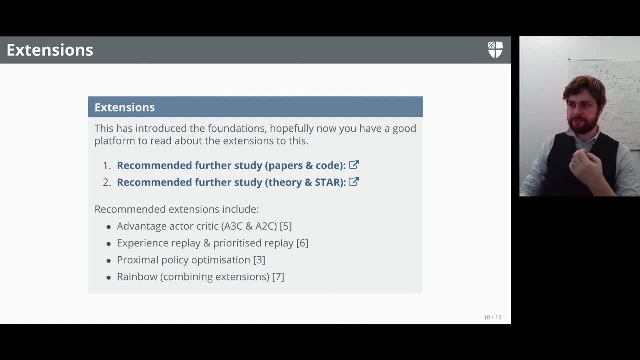 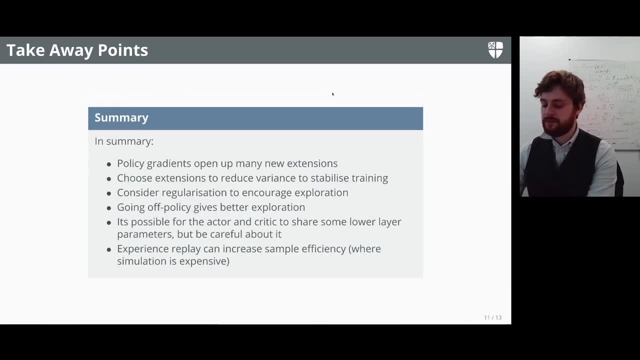 which is very good for good technique for learning advanced mathematics. So I'd recommend the Feynman Technique in just reading some of these papers here. So just oops, sorry. This first paper here is basically what we just looked at in the code. 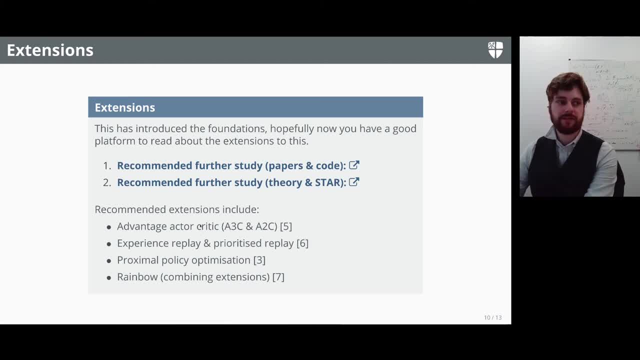 It's just that Advantage-Actor-Critique extension, So you should already have some exposure to that. But the second one here just shows that you can also add experience replay to active critic methods, as we saw in the DQN lecture last week. 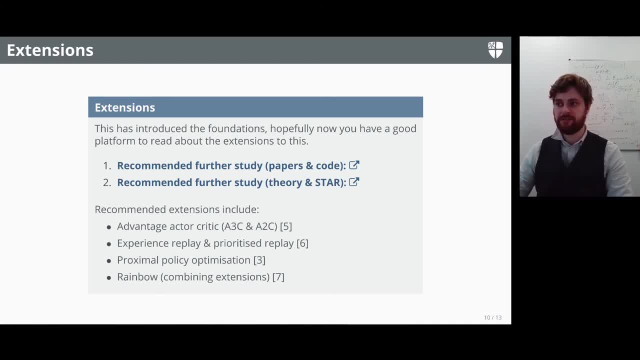 And this gives a further increase to stability and can also be used to increase the sample efficiency. So, for example, if you have like a robot that takes a very long time to perform an action, it can be better to actually train if you're using, like some replay buffer. 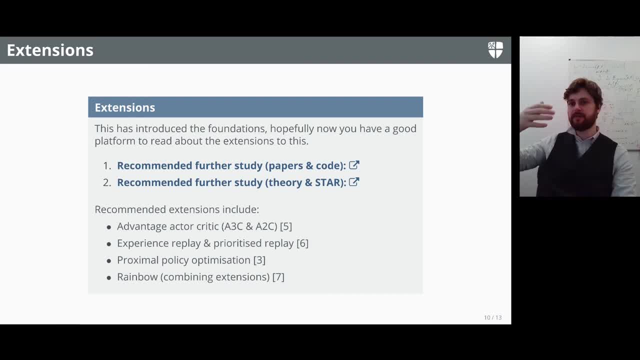 where you don't need to do all of that processing again. you can just look up those memories from your experience: replay buffer And similarly. if you find, like the CPU Atari simulation, the performance bottleneck is actually in the environment, then you can maximize your GPU occupancy a lot better. 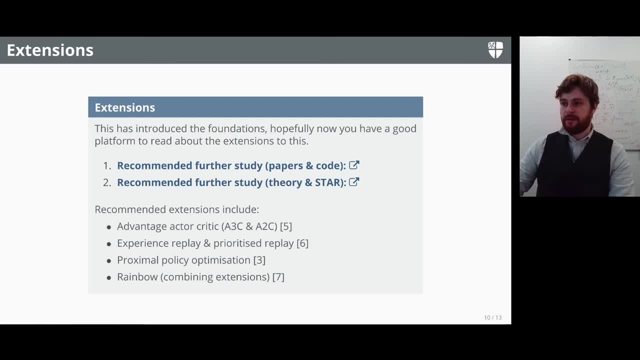 if you just store those experiences in a replay buffer, You can also do prioritized replay And again, as we mentioned in the previous lecture, where this is just where your experiences are rated or prioritized according to some puristic, And then you can sample based on those probabilities. 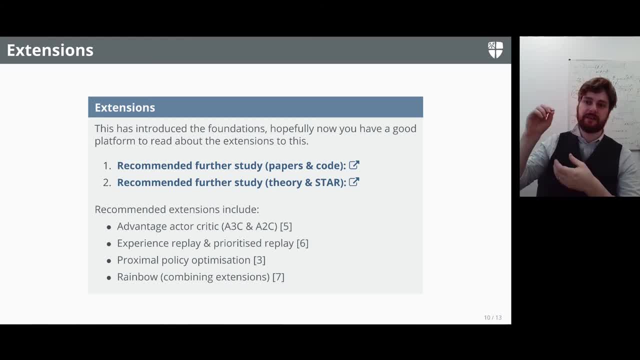 so you can use, like NumPy, that random choice to specify the probabilities from which you sample your replay buffer to learn from. The proximal policy is like a very carefully designed regularizer that can be added to vanilla actor critique methods And it can be implemented efficiently. 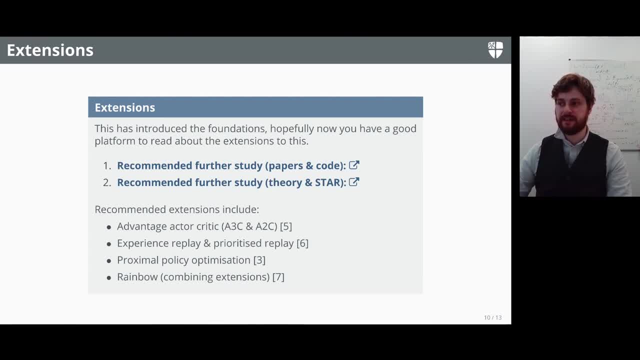 and it strikes like a good balance between sample efficiency and simplicity. And then rainbow down here is really like lots and lots of these techniques And it's this huge, so it tries to find out what combinations of all of these extensions and tricks work really well. 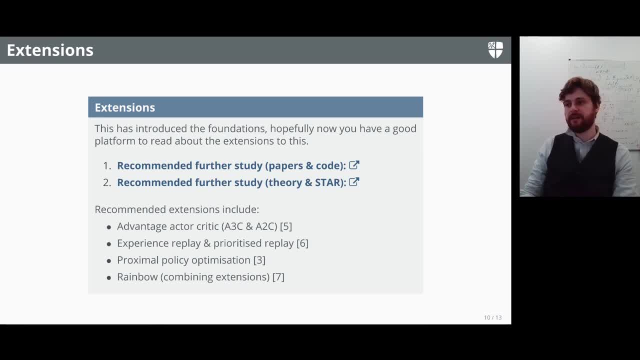 in particular for Atari. So it's basically: they've created this larger algorithm with lots and lots of combinations of them and worked out which combinations work. well, That's quite a useful paper to read, All right, so that kind of concludes this lecture. 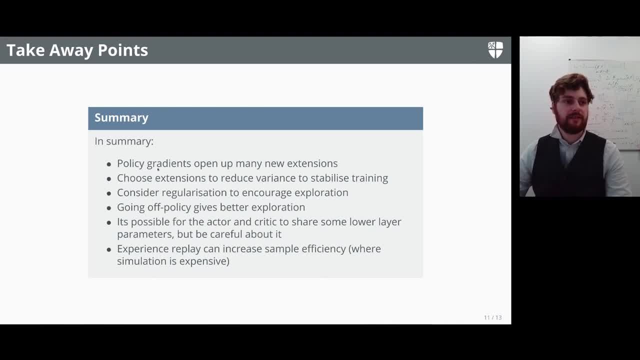 So, in summary, we've seen that policy gradients. they open up many, many new extensions and the foundations that have been taught today lead into many, many new papers around these variants where you've got this actor and this critique working together. But there are lots and lots of extensions available. 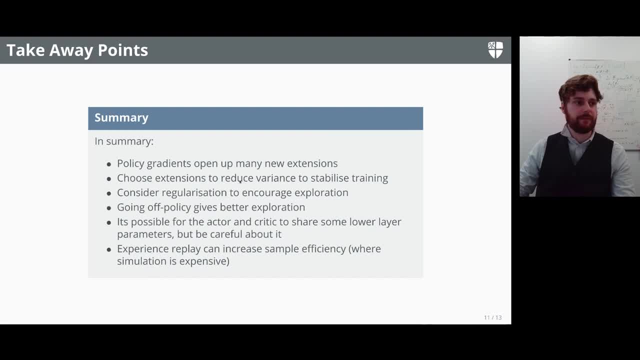 and they mainly have this bias variance trade off problem. So try to choose the extensions that reduce the variance, which helps stabilize the training overall, Because a lot of the time you get like lots and lots of noise in your optimization, as you've probably seen already in the sample code way. 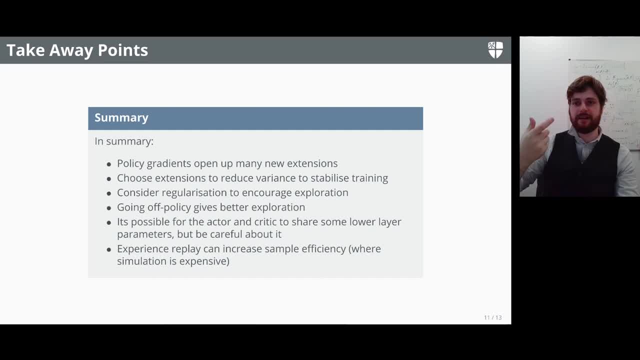 you get like one good play from randomly exploring And then most of the time, on average, you just get zeros everywhere. So you get high variance. So try to focus on extensions which reduce that variance and that makes it easier to actually train these models. 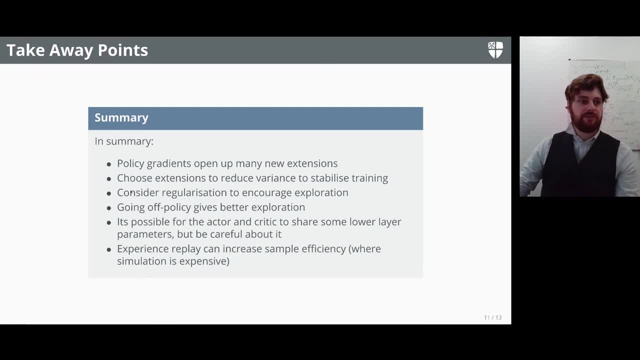 Consider regularization to encourage exploration as well. Try and do things smoothly where possible and use large replay buffers and so on and think about prioritizing them. Going off policy gives better exploration If we're just learning on the job all the time. if you remember when we talked about that. 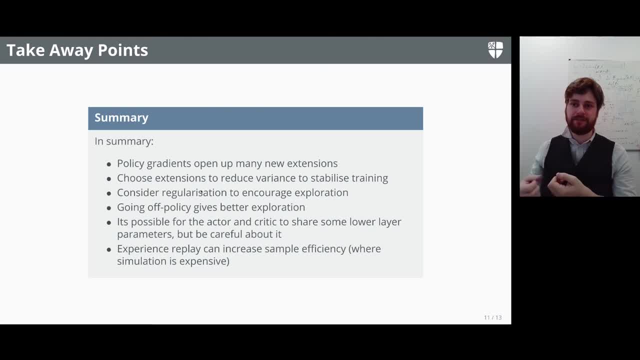 there was a few issues with that. you know, like that welder analogy where you're just thrown into this workshop and asked to weld and there's lots of things that can go wrong there. It's much better if we have this, if we're able to follow a different policy. 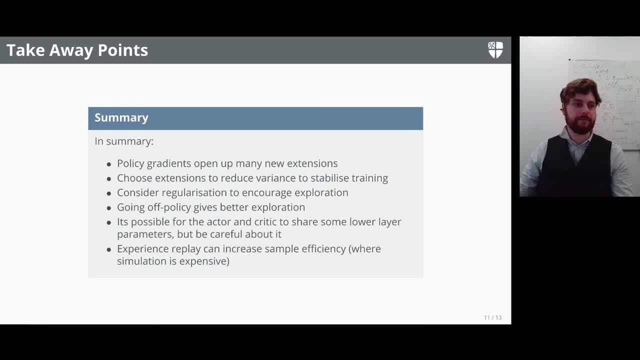 to the one we're currently considering, And it's possible for the actor and the critique to share some of the parameters, So you can actually share weights between them. But again, you have to be careful in how you do that And it can lead to a lot of problems. 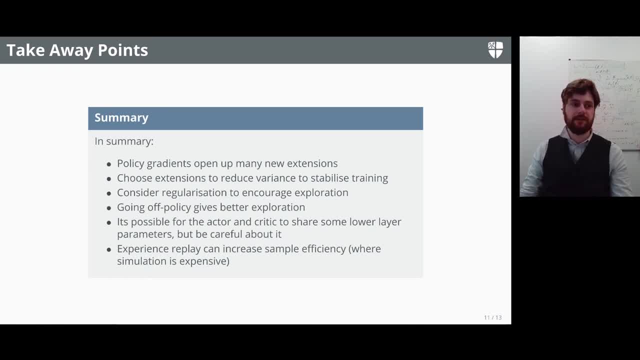 And it can lead to kind of various issues in stability if you don't take a scientific approach to doing it carefully and think to yourself: well, what's gonna happen if I start sharing these, sharing these layers and sharing these weights? So, for example, if you've got an actor and a critique, 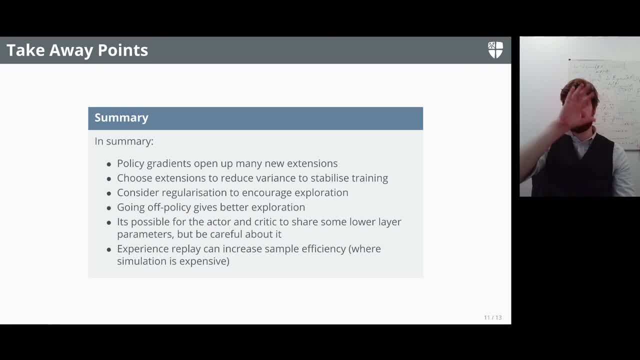 and they're taking some observations of the states, then the initial parts of the observations might be sensible to have some similarity. like the visual system of the human brain, it's fundamentally a visual system. So if you've got two humans, the way their eyes work might be similar. 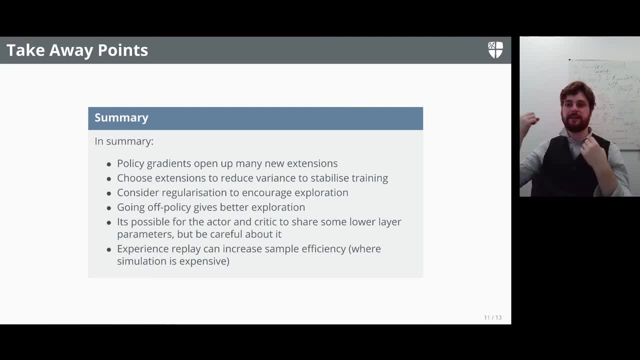 but then you want to diverge and have different behaviors for the actor and the critique in choosing the actions and judging the value. And then finally experience. replay can increase the sample efficiency in cases where simulation is expensive, So in cases where it requires a lot of processing.